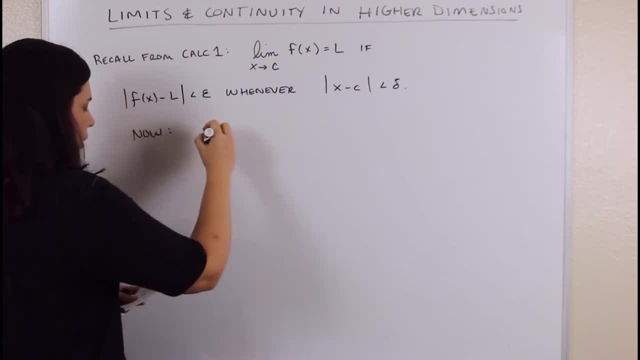 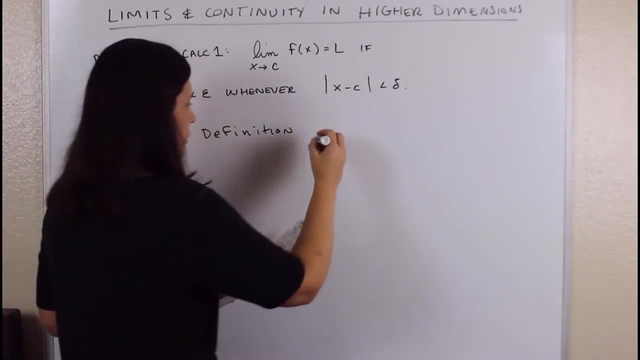 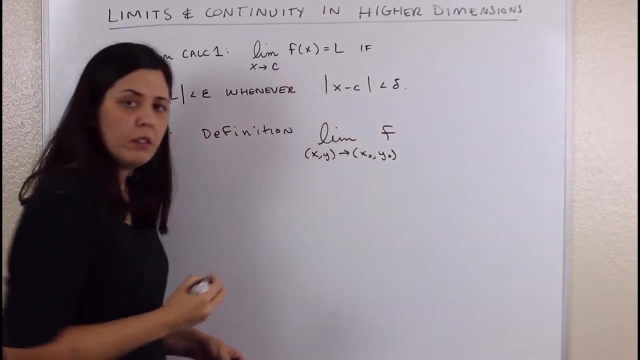 And so here's our new definition. So we'll say now: Our definition for the limit of a function of two variables is the limit. this time we're going to do x and y. So as x comma y approaches some point- x naught, comma y naught- of our function that now depends on two variables, x comma y equals L. 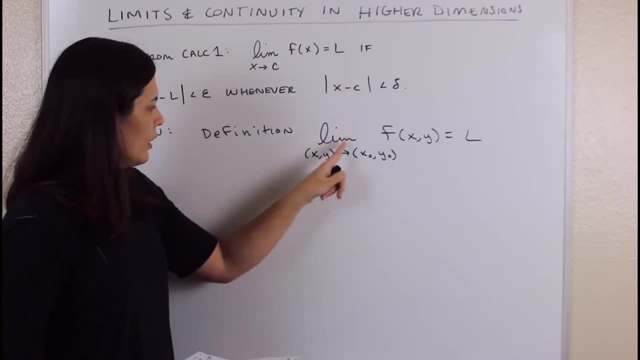 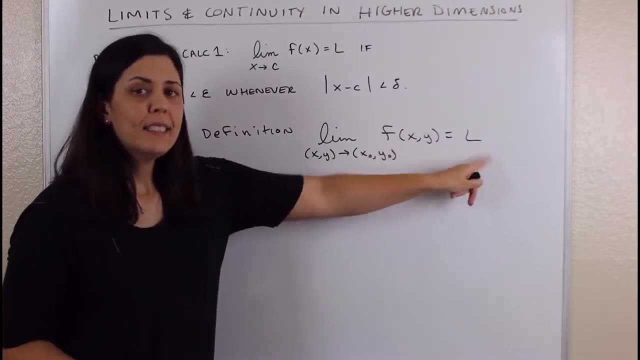 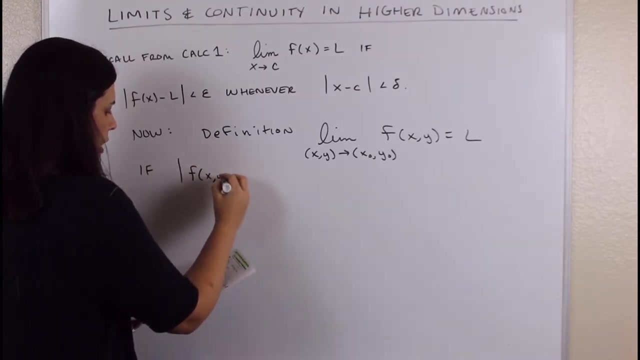 So, going from single variable To multivariable, Our limit is x, y approaches x. naught y naught Of our function, That's a function of both x and y. Has this limit value if the absolute value or the distance between f of x, comma, y and L is less than epsilon? 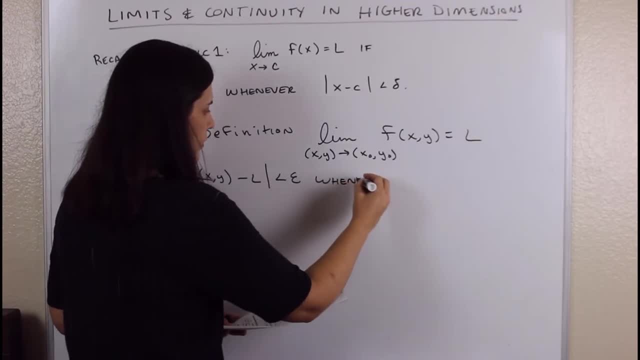 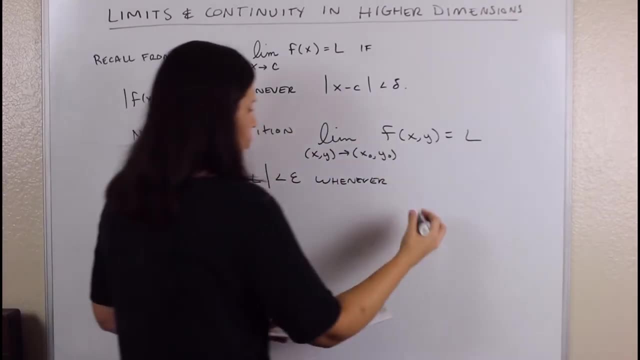 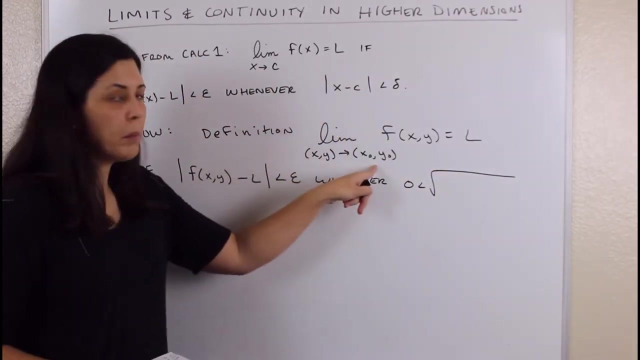 Same thing here, And this is whenever, Whenever. Now, this is where we have to think about how to translate this part, whenever the distance between this point and the point we're approaching is small. So how do I show that with a point in space, not just a regular x number, but with an 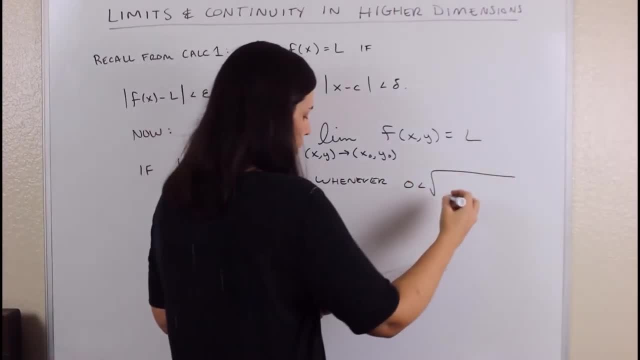 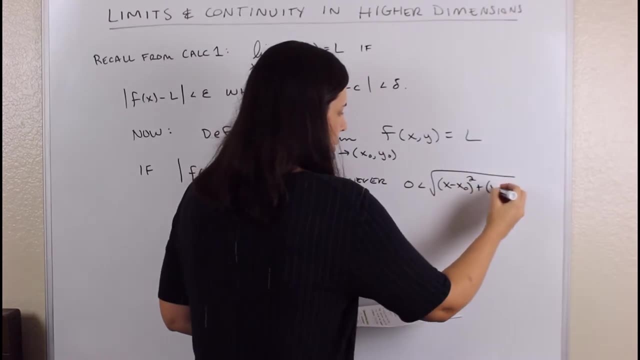 I use the distance formula, So that's what I was starting to write here with the square root, So the distance between the x components. so x minus x naught squared, plus y minus y naught squared, and this is less than delta. 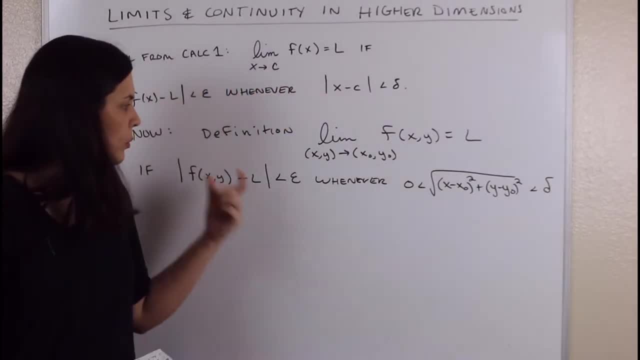 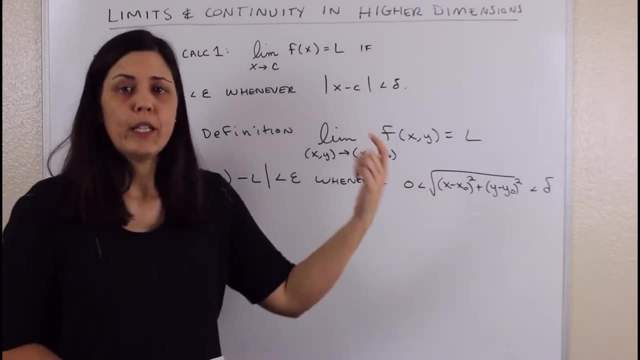 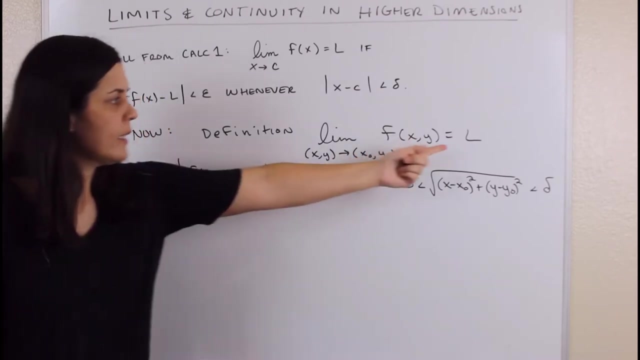 So this is just extending our single variable limit definition to multiple variables, And so what this ends up looking like visually is I'll show you. actually, you're creating what's called a disc around your point in space. that's your output, which is L. 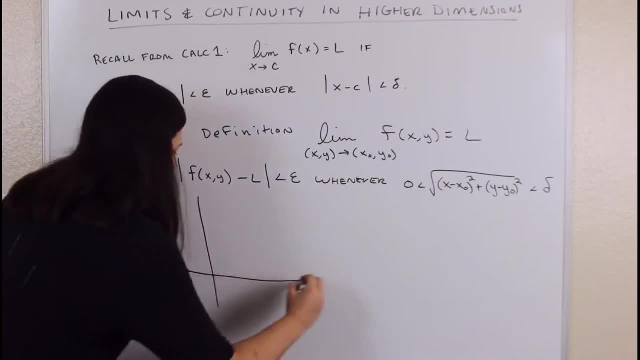 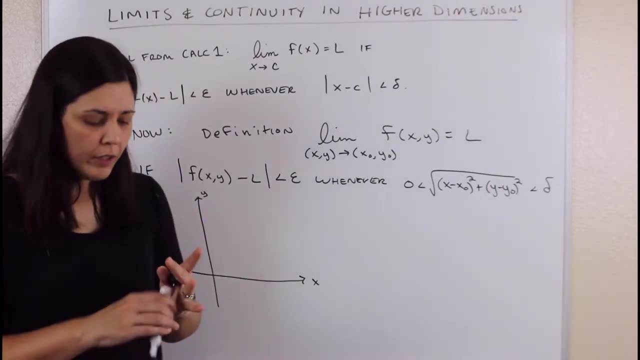 So let me show you what I mean. So we have our x and y axis And this is only our input, so this is only our domain In single variable functions. this was the input down here and this was the output here. 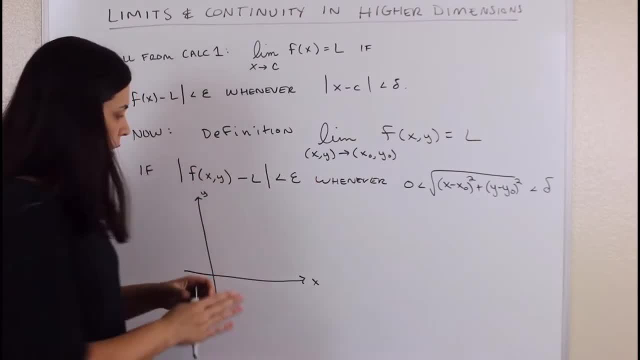 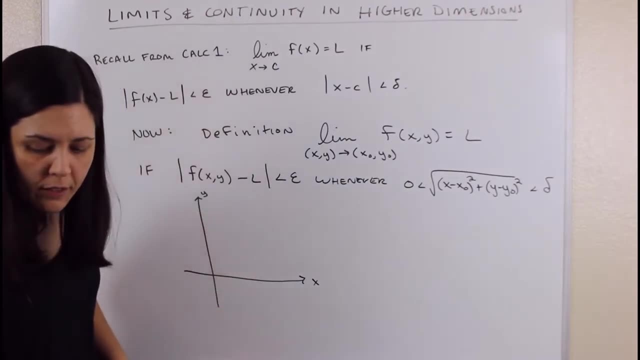 But now our output. you can call it z, So it's another dimension, like you can think of it as not even being drawn, it's coming out of the board. So all of this is just my inputs, And so visually, what I can say is, let's say, my x naught that I'm approaching is here. 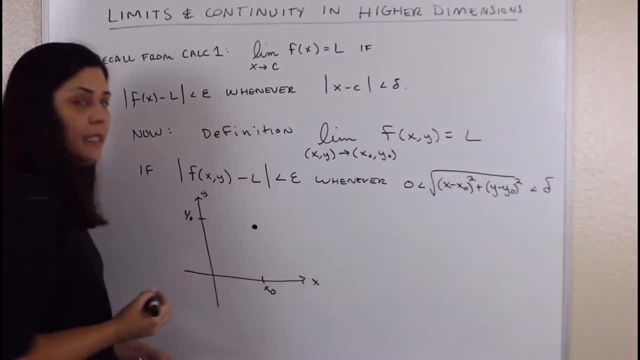 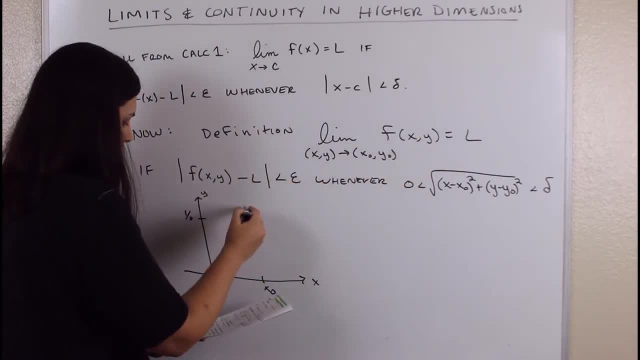 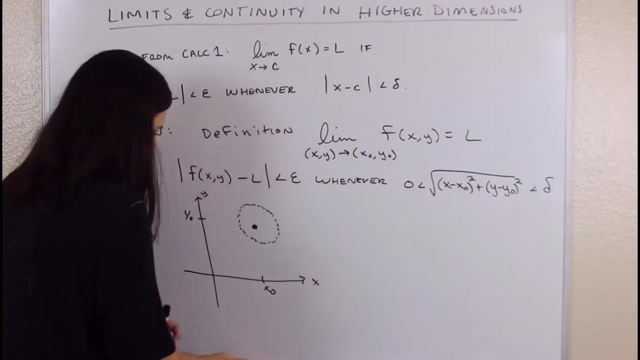 as plugging things in. Okay, And so we basically say that this limit exists, if I can create this disc around that point, And the distance between R, x, y and what we're approaching has to be small. It has to be less than delta. 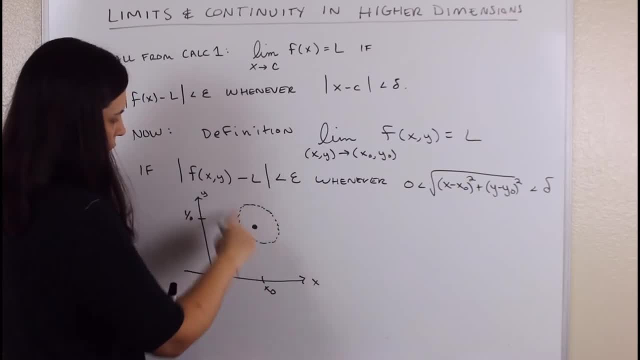 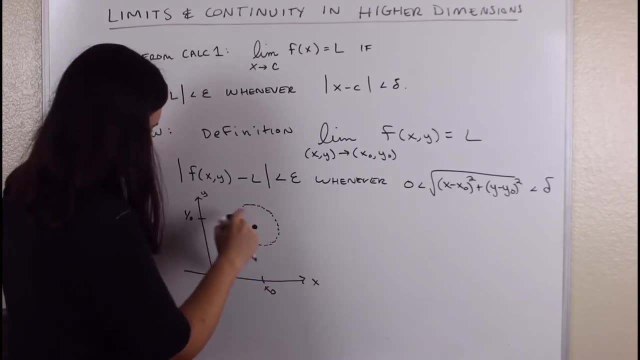 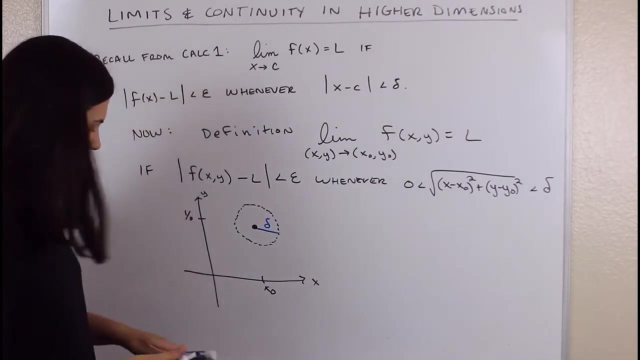 So where delta comes into this picture- and this should be more circular, like centered around this point. My drawing's a little off. Let's make it slightly better, Okay, Okay, here this delta is. here it's actually the radius of this circle. So instead of just 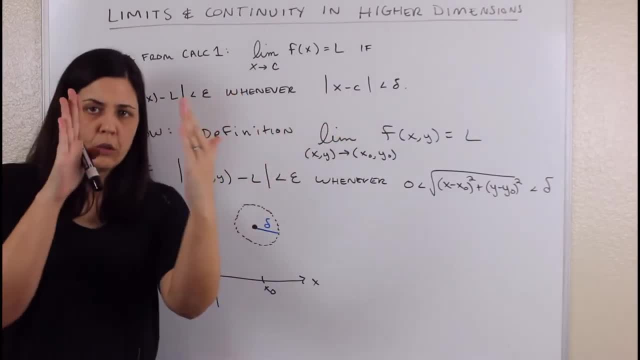 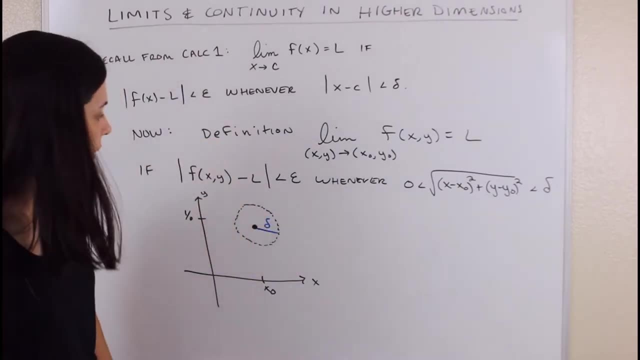 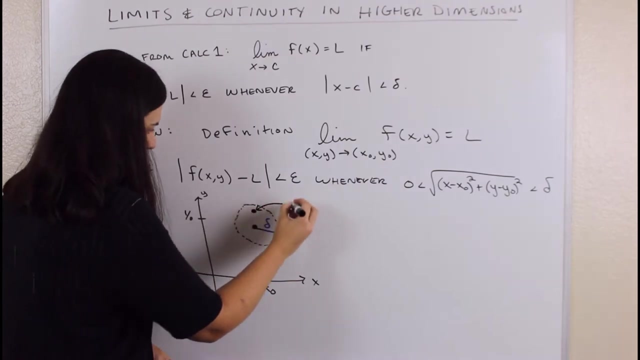 sticking to just the x-axis and staying within the delta range on a single axis. I'm staying within a delta in terms of x and y, so that's why it's the radius of that disc, And so when this happens, so let's say our point is here, so we'll say that that right there. 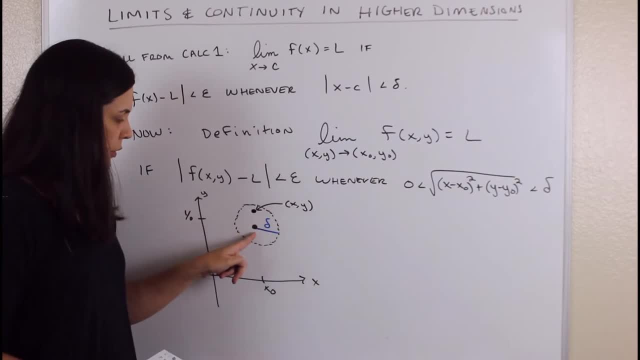 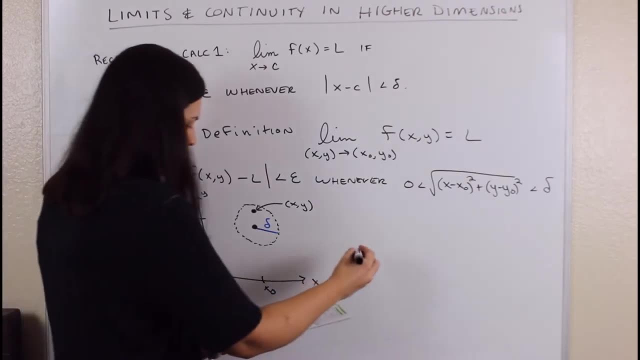 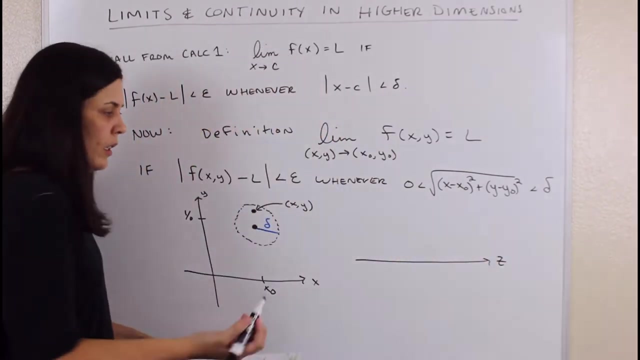 is x, comma y, but it's close enough to what we're approaching because it's less than this finite distance away. When that's true, then our outputs: we'll graph them on a separate axis, I'll call it z. so our outputs are really close to L. so let's say this is my L value. 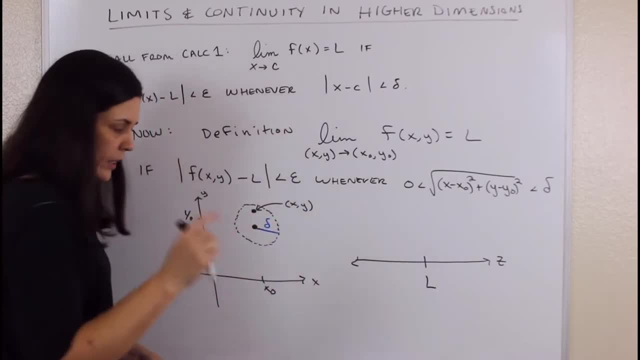 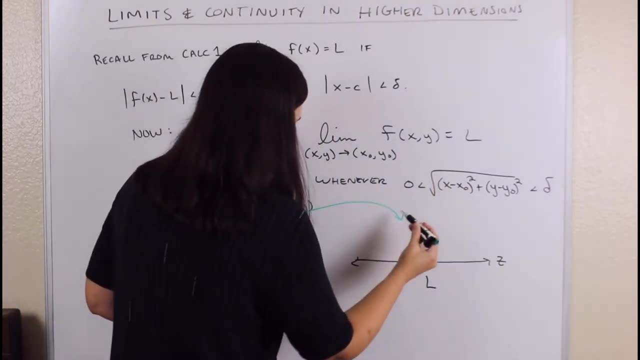 my f value. so if I plug in. so stick with me here- if I plug in this point into my function, it's going to be 0.. function x comma y, then my f of x comma y. it's really close to this limit value. 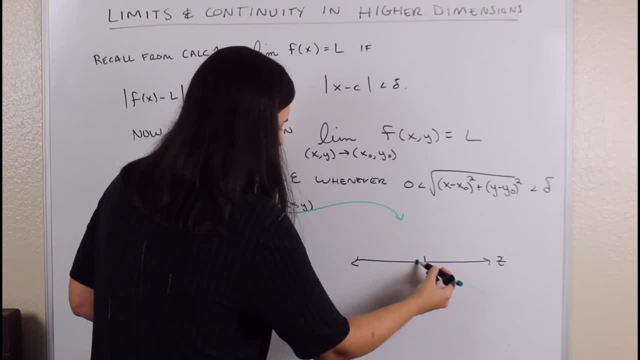 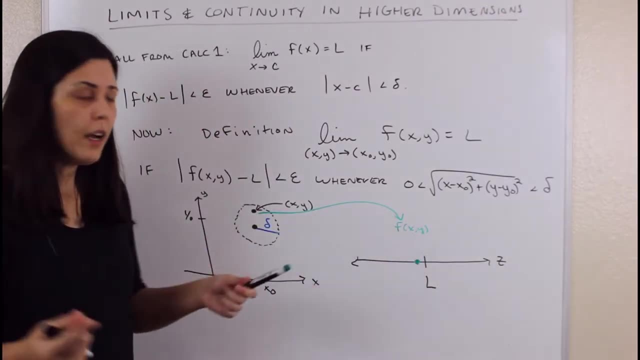 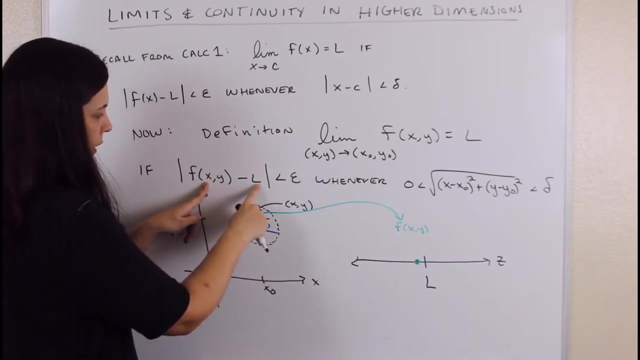 It might even be that limit value. I'll just make it different to show you what I'm saying. So this right here is f of x comma y, But it's close enough to L because this part here is saying that the distance between this output value and my limit is really small. It's less. 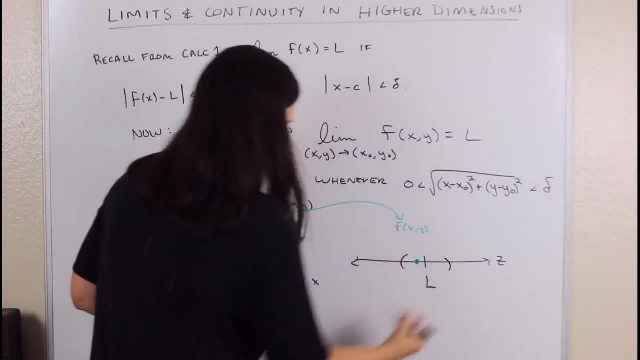 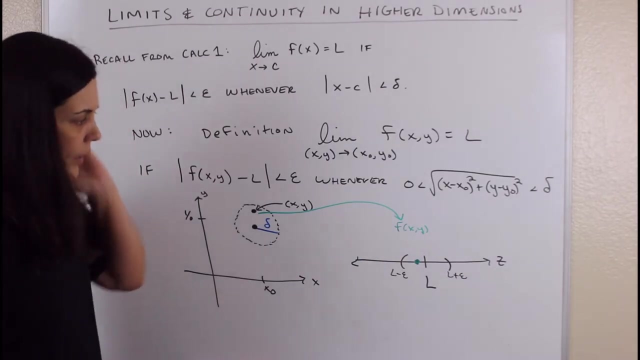 than some arbitrarily small number, epsilon. So this right here is epsilon and epsilon. So this is like L plus epsilon and this is L minus epsilon, And we're within that range or interval. Alright, so this is the formal side of it, just to show you the definition. 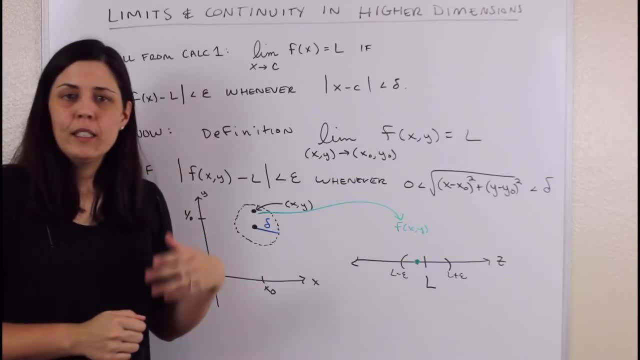 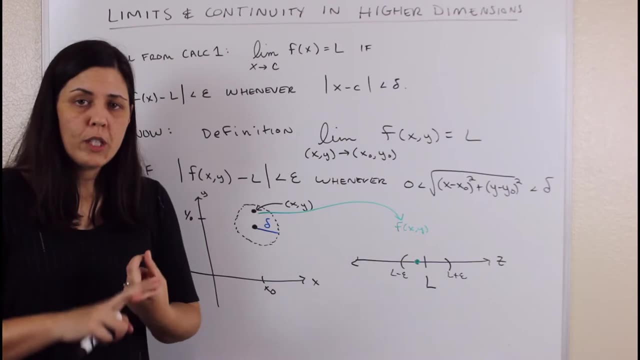 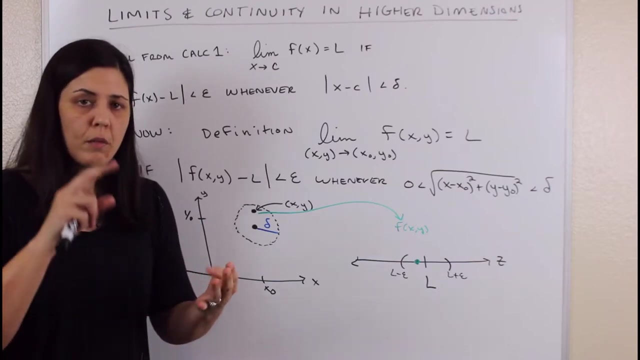 of our limit in higher dimensions. But the nice thing is, everything you know about limits from single variable functions, it's still going to work. So your sum difference, constant, multiple rules, radical power, all those limit rules that you've learned way back when you started calculus, they're still going to work here. 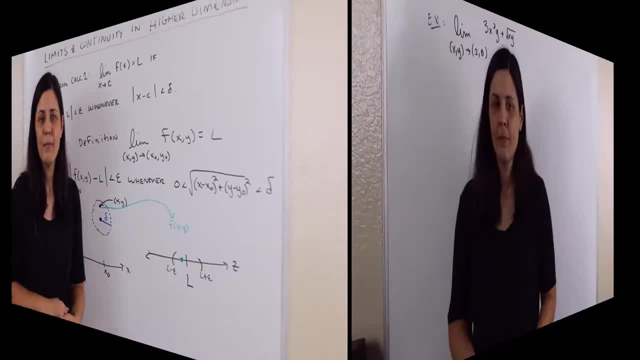 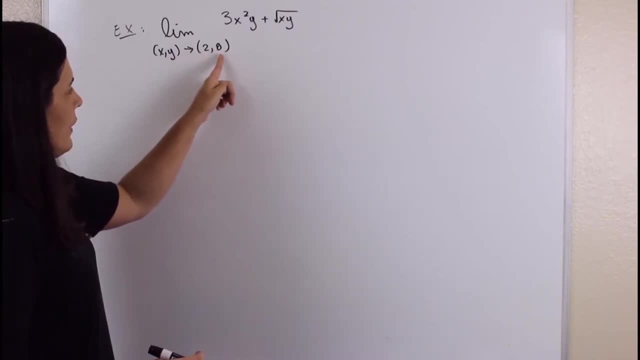 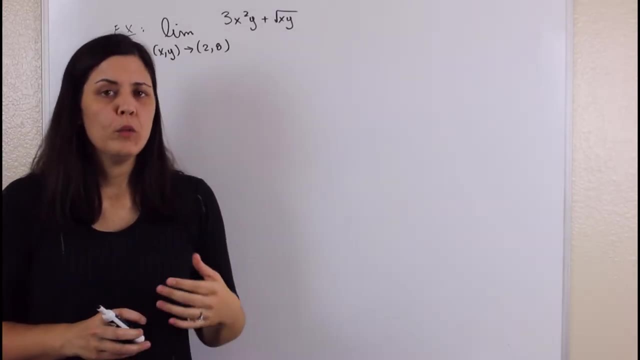 So let's just jump right into it and work out some examples. Okay, so here's this first example. Find this limit as x, y approaches 2, comma 8 of 3x, squared y plus square root x times 1.. Now, if you remember when you first learned about limits, what you want to try to do is: 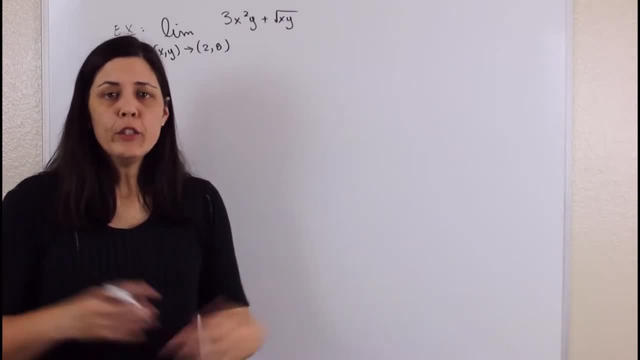 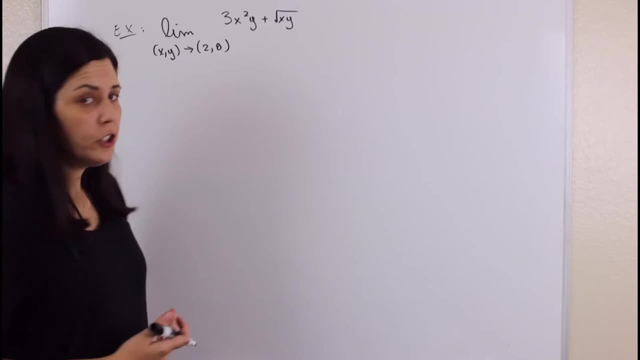 just direct substitution. If that doesn't work, then you try something else. You try some other techniques that you learned- and I'll show you a different example to use some other techniques. But let's jump right in and see if direct substitution works. 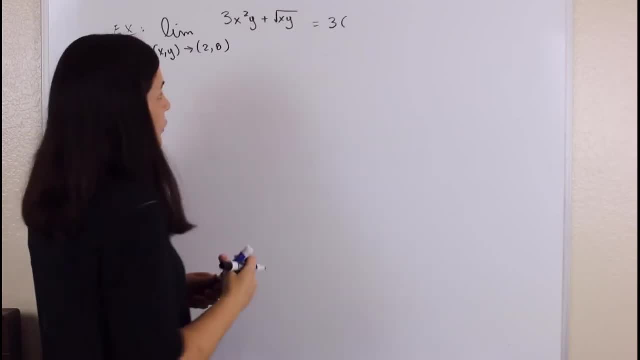 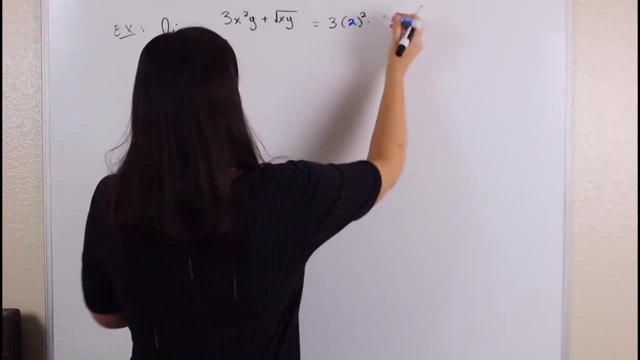 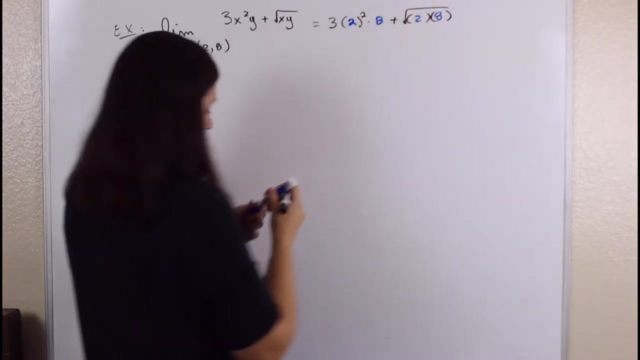 So if I just plug in my values for x and y, let's see if we get a real number answer. So x is 2, so 3 times 2, squared times y, which is 8.. Plus square root of x times y, so that's 2 times 8.. It's looking good, There's nothing. 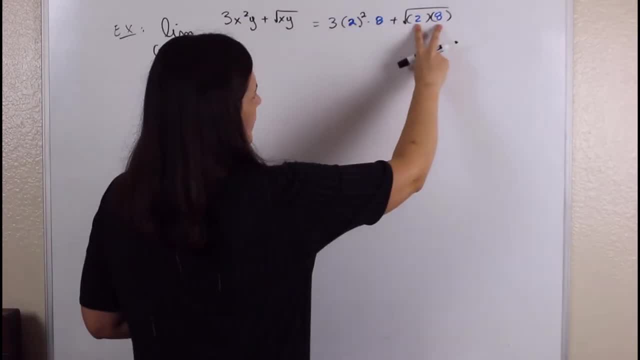 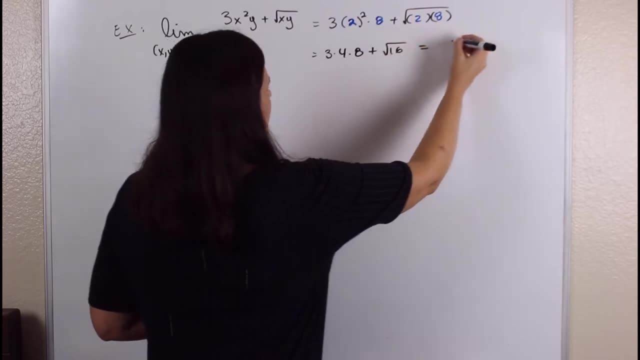 that's going to make this undefined or not real. This is positive inside the square root. So this is just 3 times 4 times 8, plus square root of 16.. So this is just going to be 96 plus 4,. final answer: 100.. 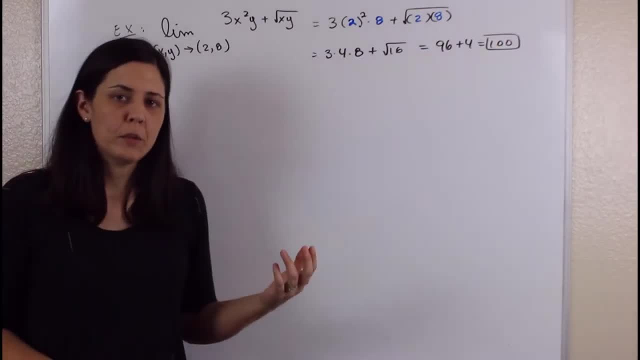 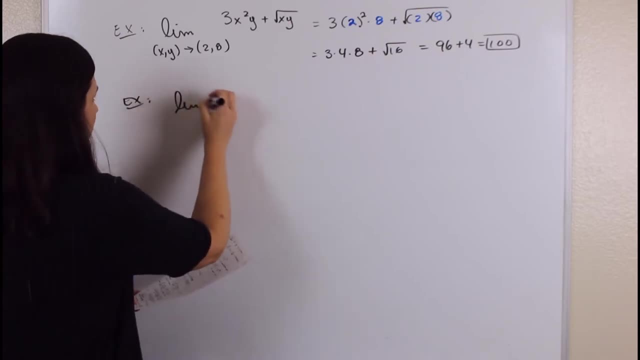 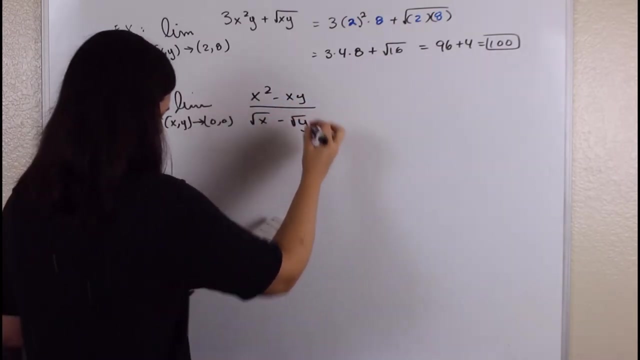 So that's it, Really straightforward computation. because direct substitution worked. Let's try another example. Let's try another example where direct substitution won't work. So the limit as x, y approaches 0, 0 and our function is x squared minus x, y over square root x minus square root y. 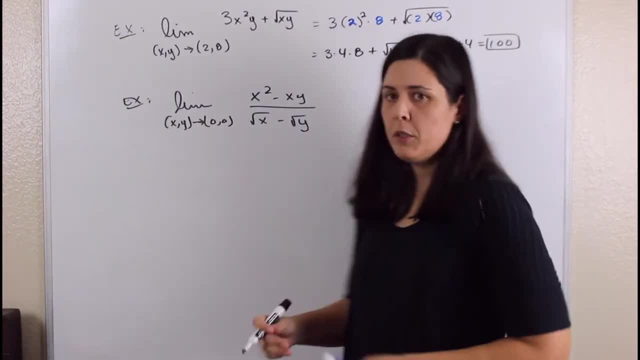 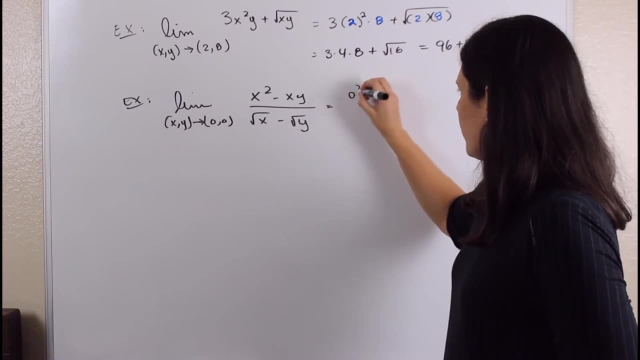 So if you can see it, you can just say direct substitution won't work and then move on. But let's say you don't see it and you just need to try. If we plug in 0, look what we get: 0 squared minus 0 times 0 on top: square root of 0 minus square root of 0 on bottom, 0 over. 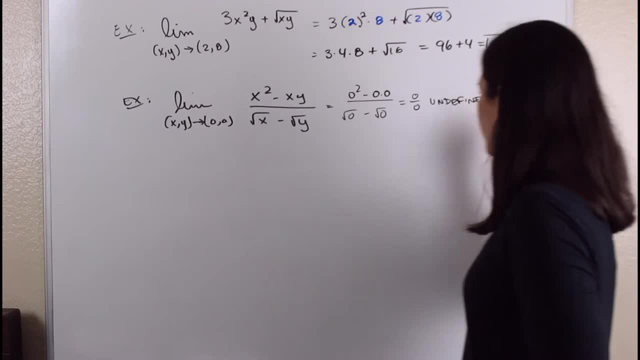 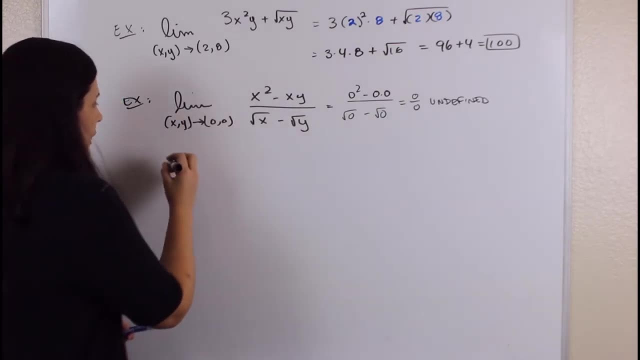 0,, which is undefined. Alright, so we have to try something different. now, If you already know we needed to try something different, you can skip that step. So, in this case, what we're going to end up doing, and if you kind of remember some of 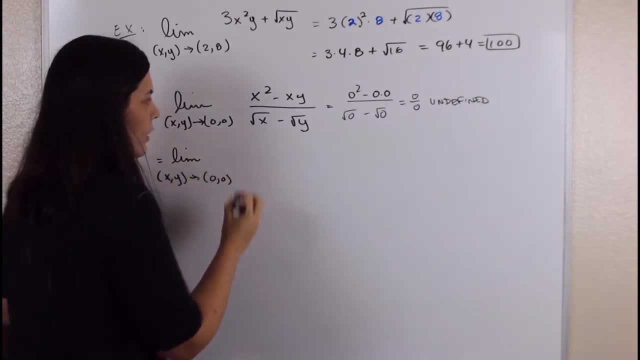 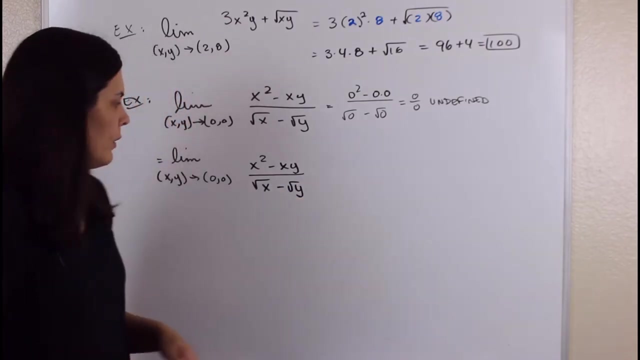 the techniques you learned when you first were learning about limits. one of them was to multiply by the conjugate of either the numerator or denominator. So I'm going to rewrite this function and then you take a look, think about it. What am I going to pick? and take the conjugate of it, The denominator. so the ones the radicals. 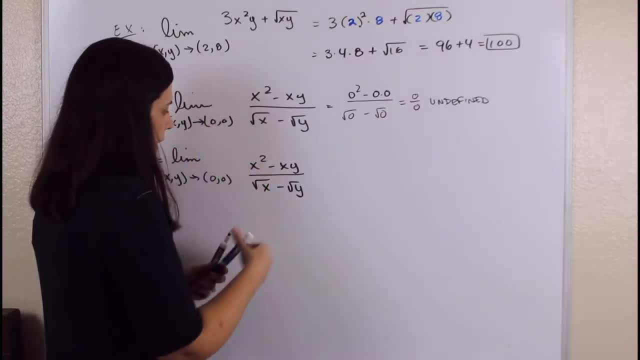 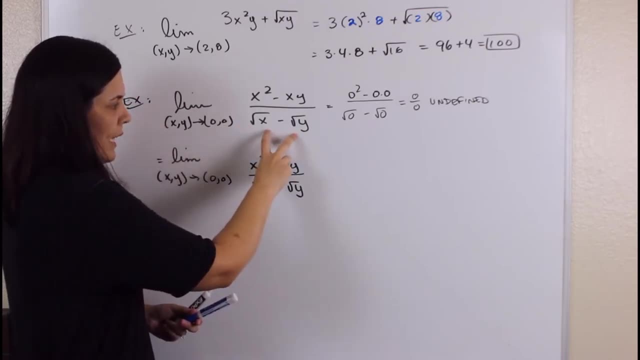 usually, and it is because I'm trying to actually get rid of the problem. And the problem is, if I plug in 0, 0, now double this combination of x and y is going to make the bottom 0, which is what makes them undefined. So I'm going to multiply by the conjugate of the denominator times the top and bottom y, which is going to make the bottom 0 and again the unit as a right stuff. This should make sure that we know that this is what we do before. So this isn't the end of the experiment. So first of you start out on your first centimeter. 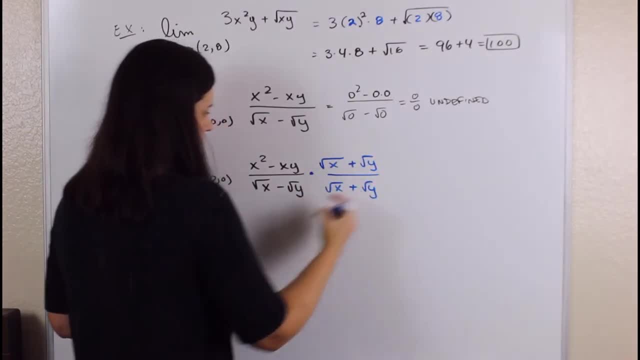 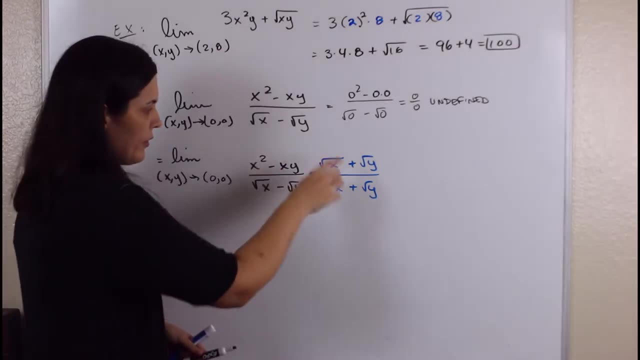 and bottom. So remember the conjugate. you just change the sign in the middle. So for us that's going to become a plus sign And now working on some algebra skills, So we are going to have to FOIL this out. But what I have learned with trying these problems is sometimes it's better to wait. 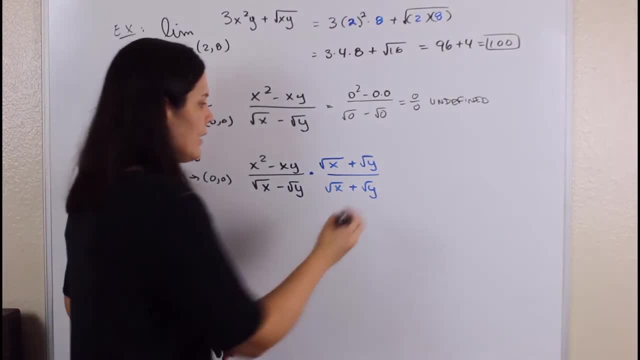 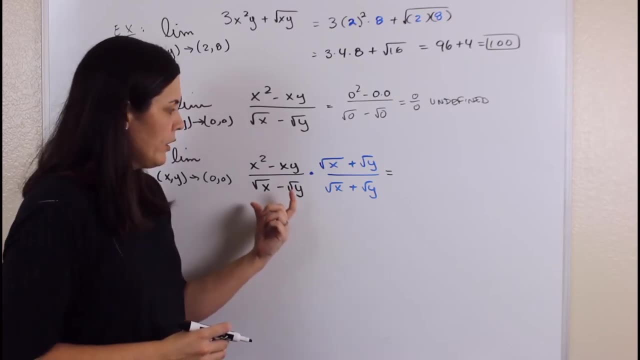 for FOILing both the numerator and the denominator, and it's going to pay off on this one. So, normally, which one you definitely want to FOIL out or multiply is whichever one you picked to take the conjugate of. So what I'm saying is: let's FOIL the denominator but leave the 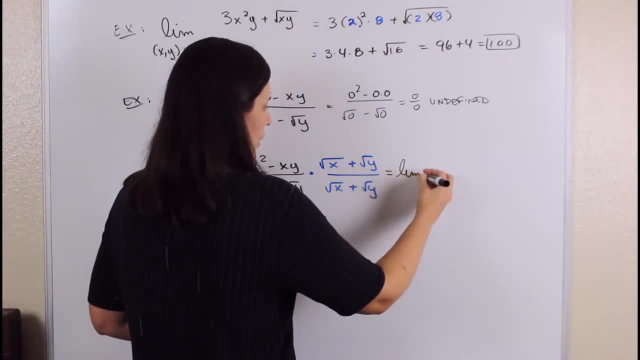 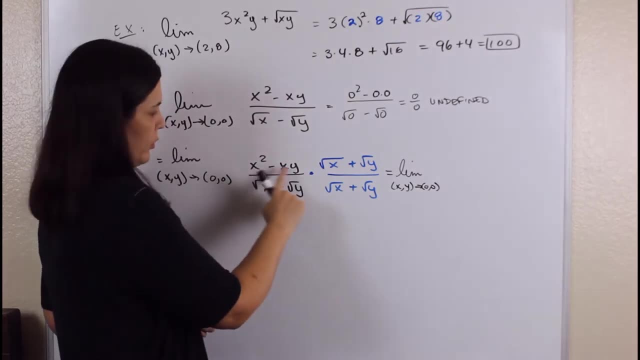 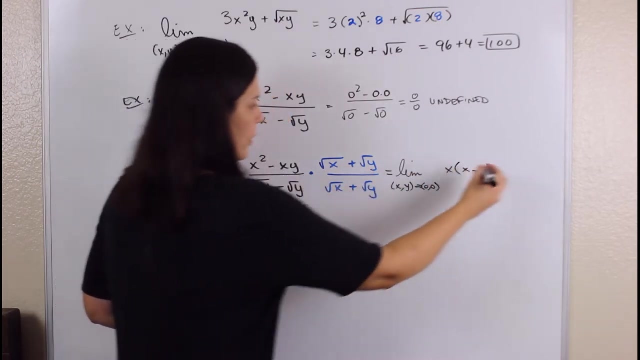 numerator factored, And so for this one I'm actually going to even factor further the numerator And so, if you notice, you can take out an x from these two terms. So my numerator is going to be x times x minus y times what we multiplied by square root x plus square root y. 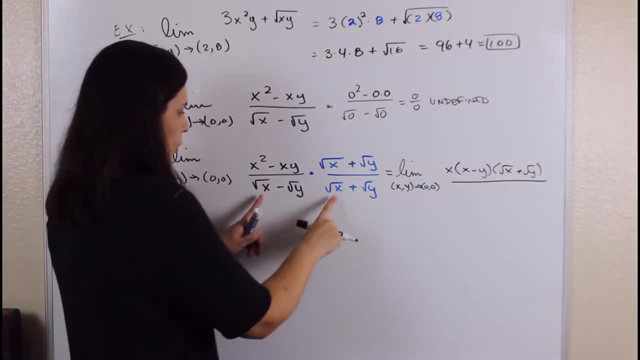 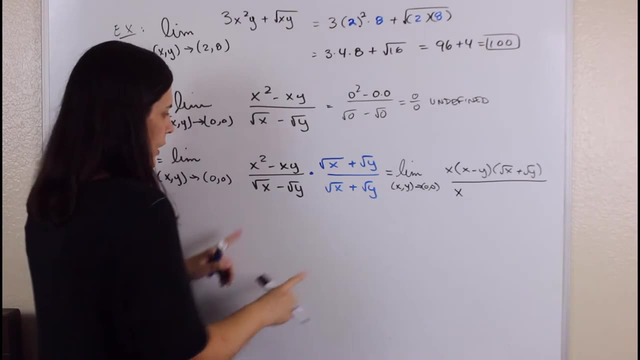 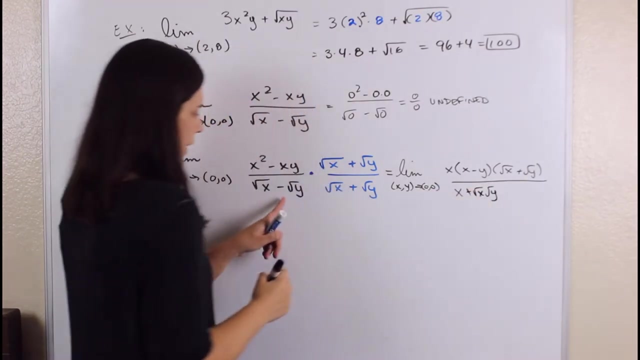 And then I'm going to go ahead and FOIL out the denominator, And so we have square root of x times itself. So it got squared, So that just became x. You undid the radical. Then you get positive square root y times positive square root x, And then you have negative square root y times. 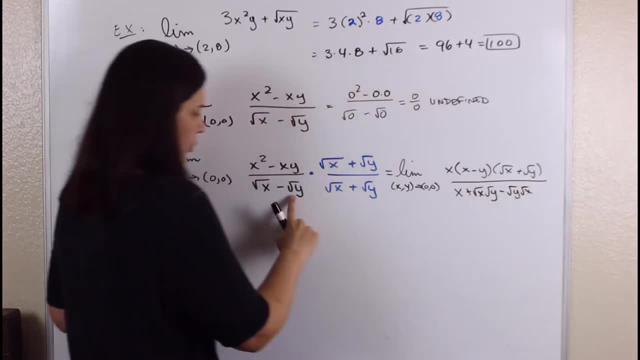 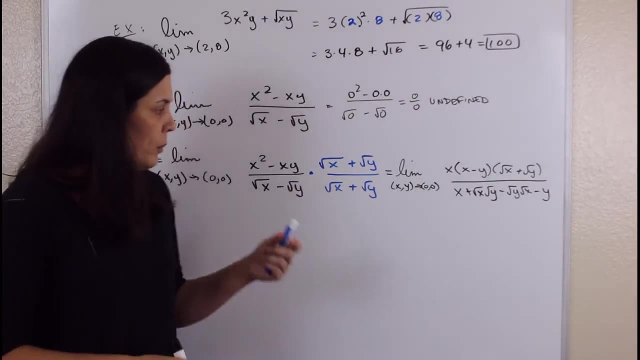 positive square root x, And then you have negative square root y times itself, So that radical gets squared away there. Now, anytime you multiply, something times its conjugate. this is always like a nice place to check if you did your work right. 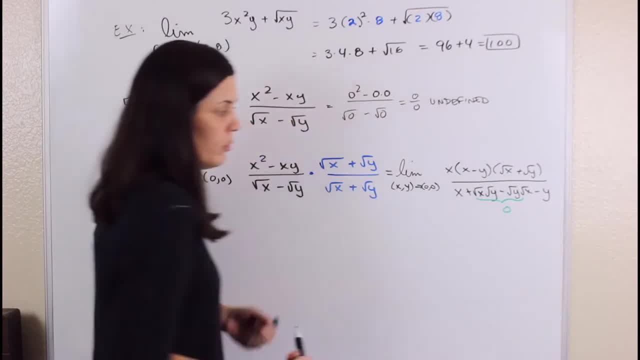 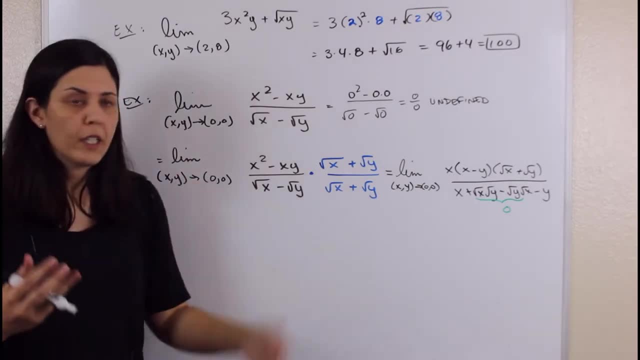 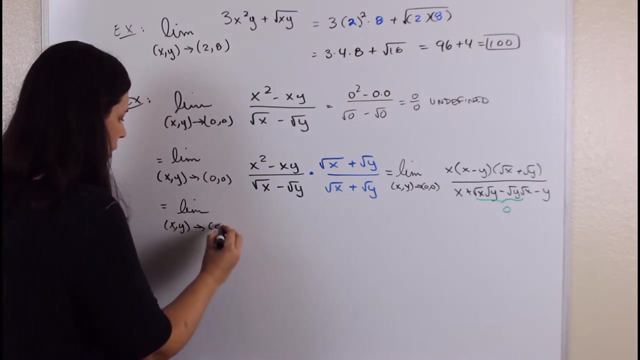 The terms in the middle should add up to zero, And these do, Plus these radicals, being multiplied minus the same thing. So that's how I know I'm on track. I did my multiplication correct, So now let's see what we get. So our limit as xy goes to 0, 0.. And on top I still have the same numerator. 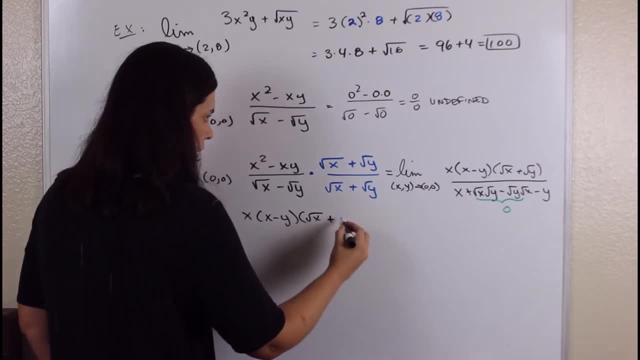 I didn't change that yet. On bottom, if I get rid of all that stuff in the middle, I just have an x minus y. And then here's where it's good to notice that we did the right thing to wait on foiling out the top. 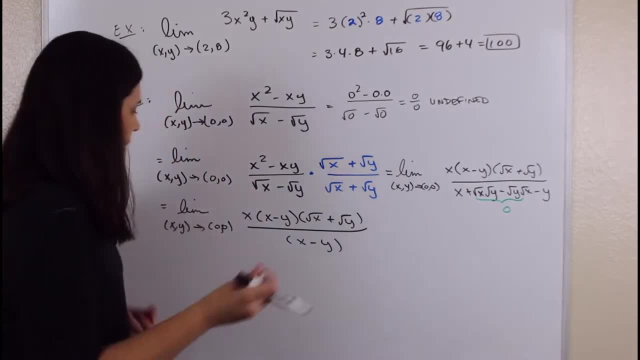 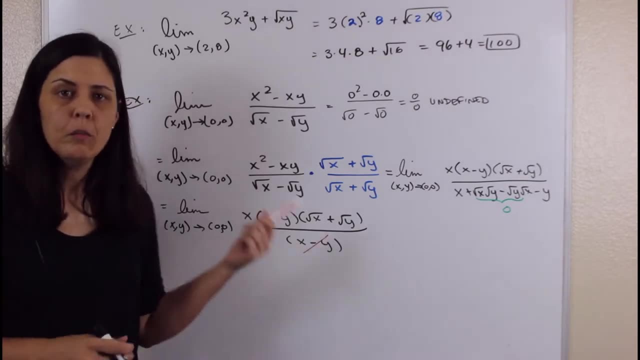 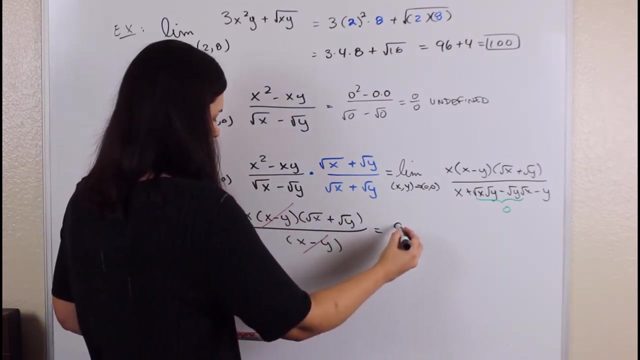 Because right here these terms divide out, And that's good, because that was the problem. The problem was, when I plug in 0, 0, the bottom was 0. So now I'm just left with the numerator. Let's go ahead and plug in 0 for x and 0 for y. So this is 0 for x times square root of 0 plus square. 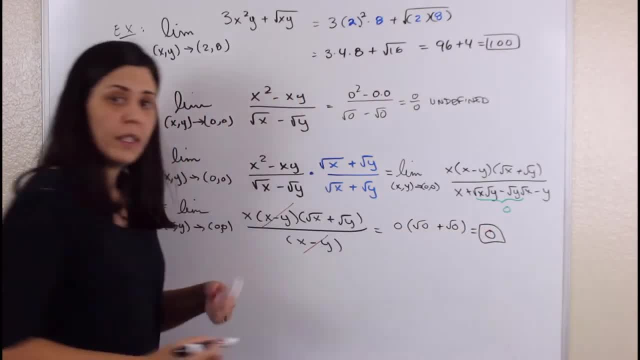 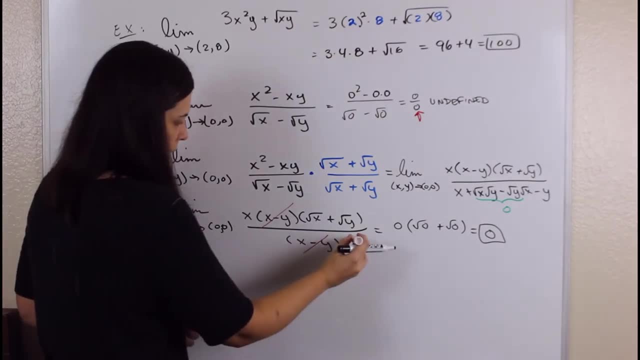 root of 0. Which the answer is 0. But the reason why this is okay and earlier it wasn't okay is because you can't ever divide by 0. And at this moment the denominator is a nice invisible 1.. This is really over 1.. 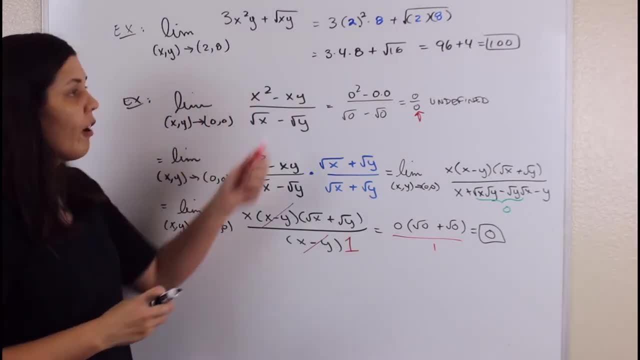 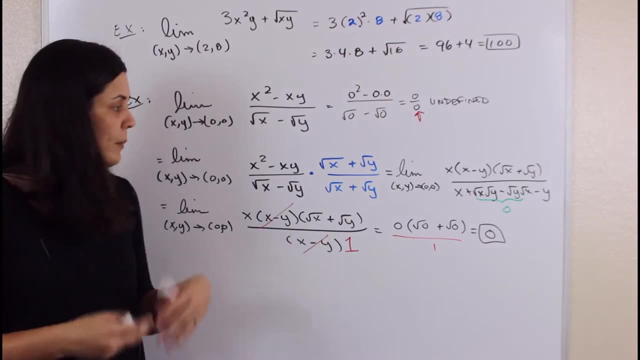 Okay, So the new part is just the fact that our function was a function of both x and y, But everything else is things that you've learned for limits in the past and just using some algebra techniques. Okay, let's keep going. So we actually have to consider the following: 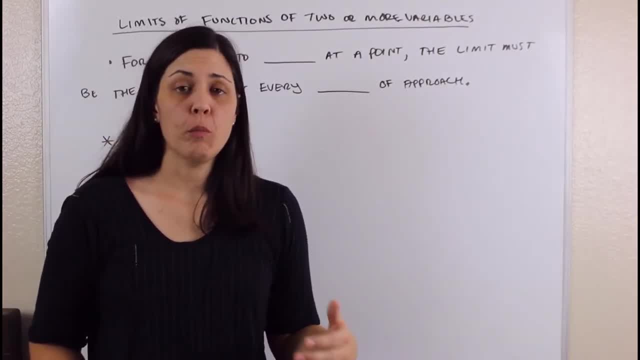 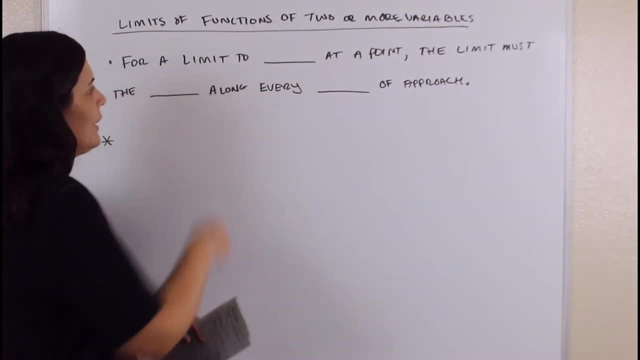 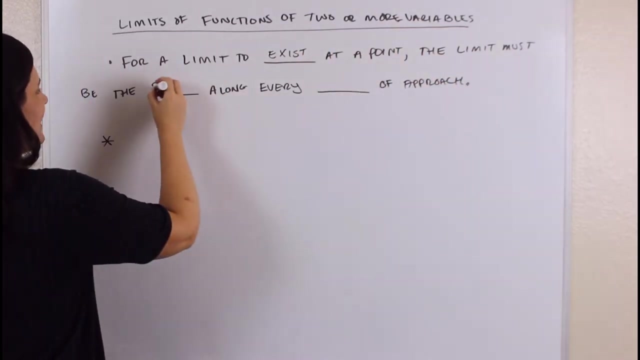 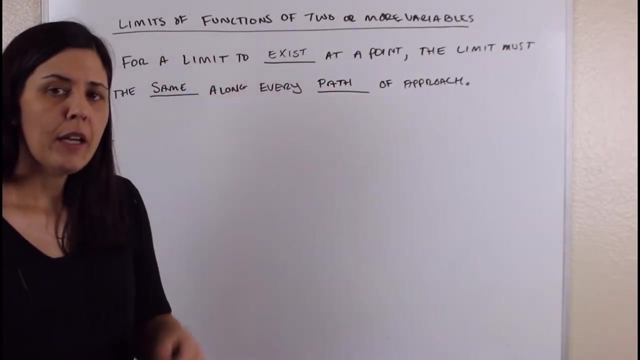 We have to consider more when we're thinking about these functions in more than one variable, And so limits of functions in two or more variables. there's more involved here. So for a limit to exist at a point, the limit must be the same along every path of approach. 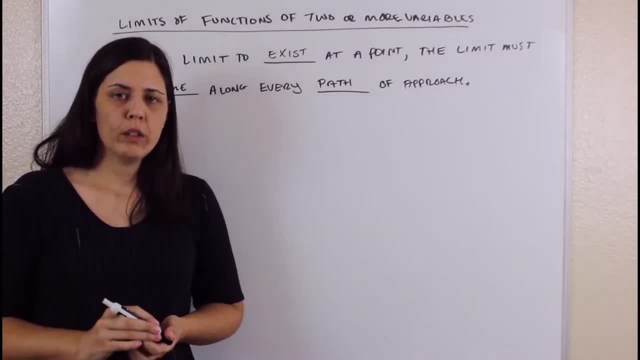 Now you know this from single variable calculus. But now that we're working with multiple variables, we're going to have to consider more. Okay, So for a limit to exist at a point, the limit must be the same along every path of approach. 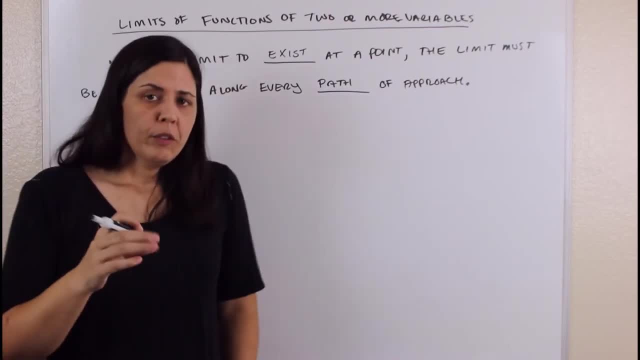 Now you know this from single variable calculus. But now that we're working with multiple variables, we have to consider multiple paths. Here's what I'm saying In single variable calculus. we'll just sort of look at it real quick off to the side here. 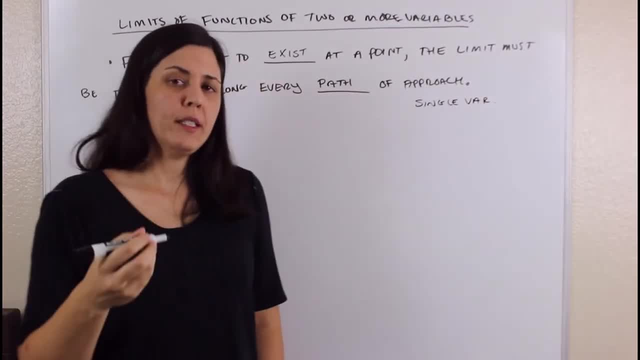 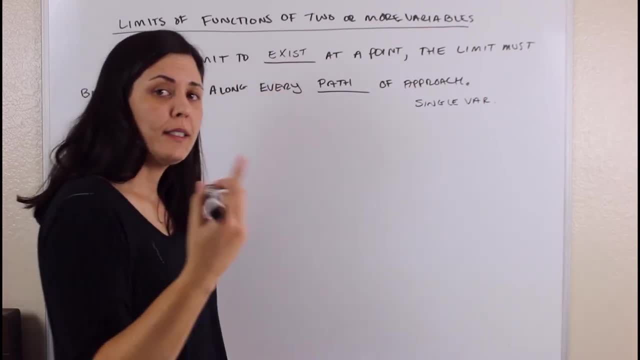 So single variable. You had to make sure two things happened, If you kind of can think back what I'm getting at. So the limit existed. if something was the same, which limits were the same? It was when you approach from the left. 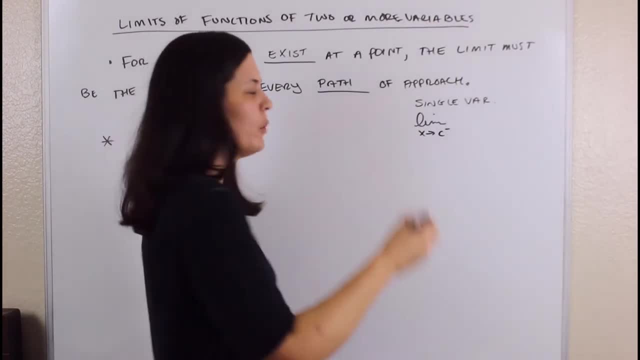 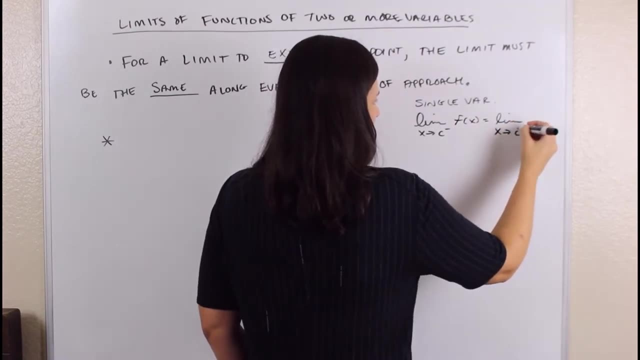 So I guess it's just one thing happening. These have to be equal. Approaching from the left Had to be the same as what you get when you approached from the right, And that was because there was only two directions or paths of approach. 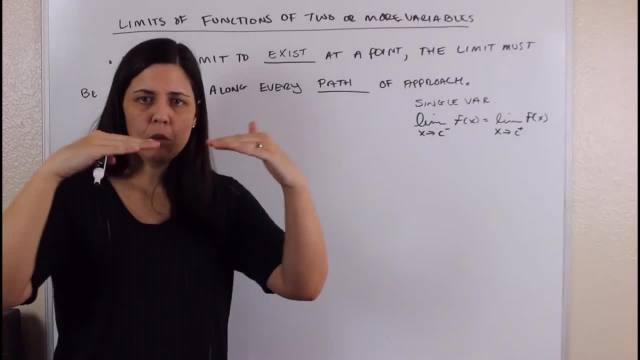 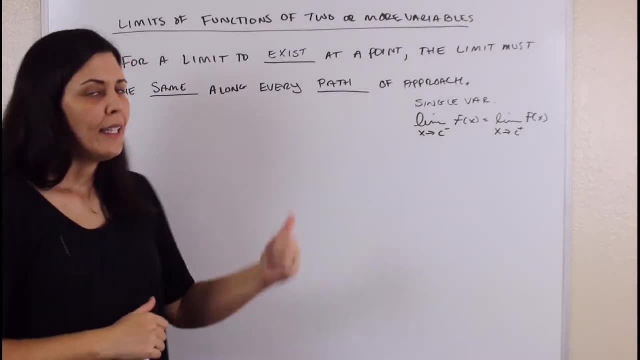 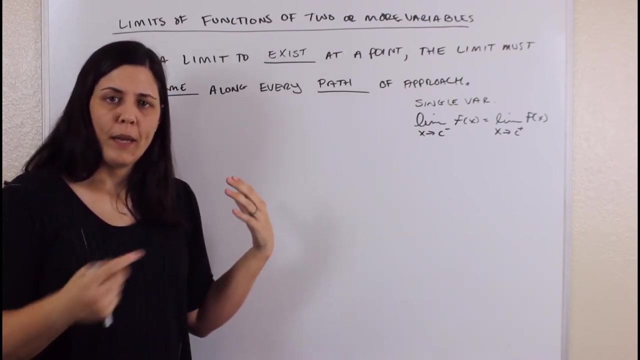 I can approach from the left or the right of my x number because it was a single variable It was only focusing on, like the x axis, So that's all I had to make sure of. Now I can actually approach from any direction. If you look kind of think back on our drawing we had with the domain the x comma y. 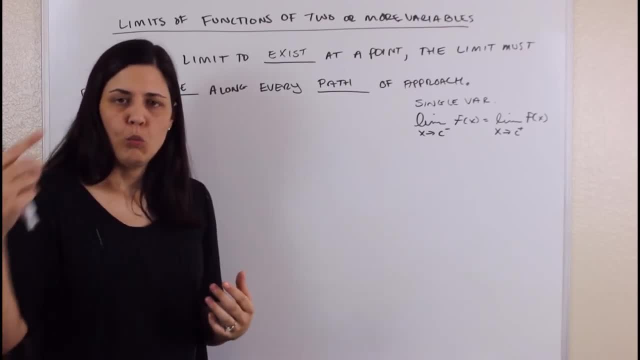 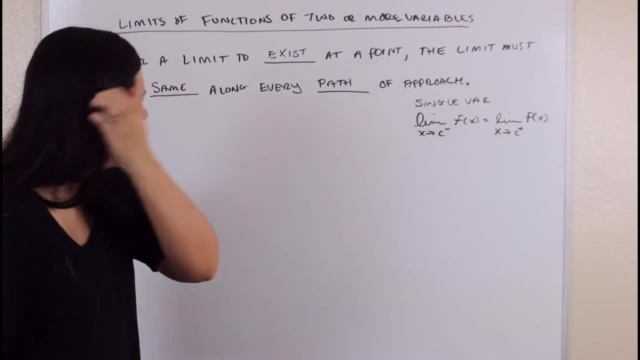 I can draw all kinds of paths to get to that point. It's not just one left and right path, It can come in from the top, from the bottom, the side, at an angle, curve, straight, all kinds of things. 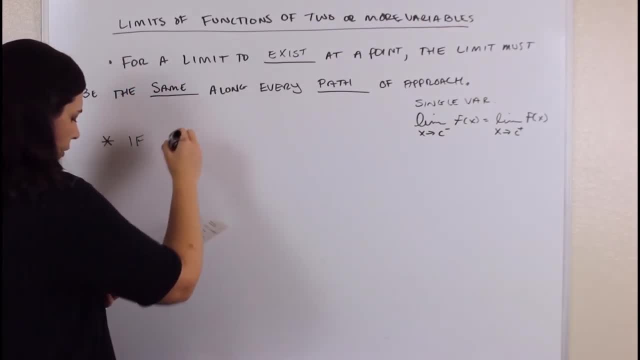 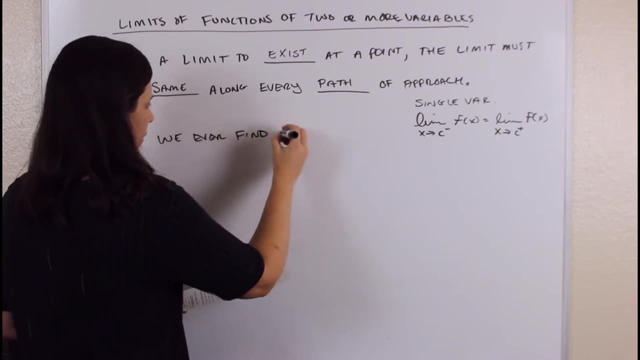 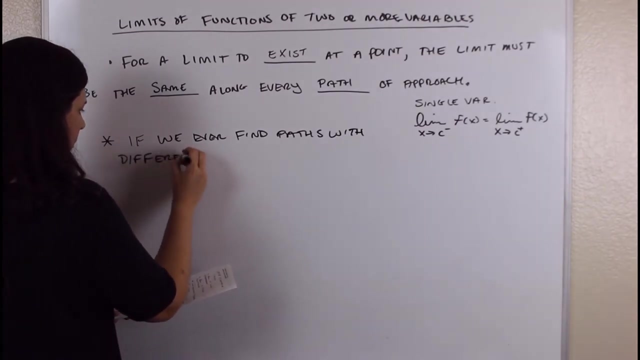 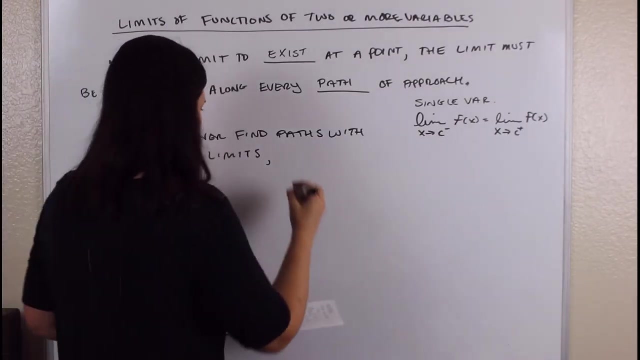 And so what we have here? well, let's first say this: If we ever find paths with different limits, So if we ever find paths with different limits, Okay, Okay, Okay, Okay, Okay, Then the function has no limit at the point they approach. 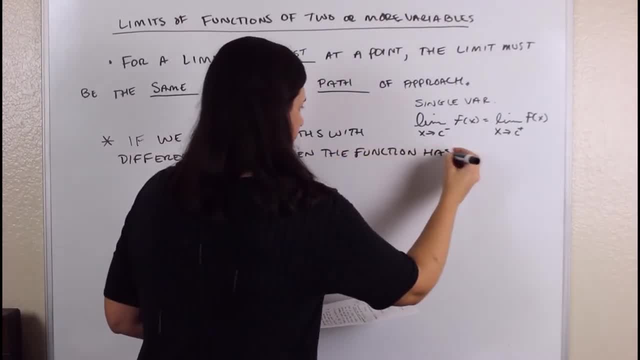 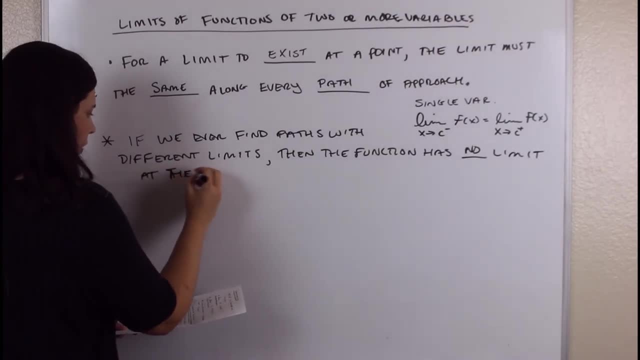 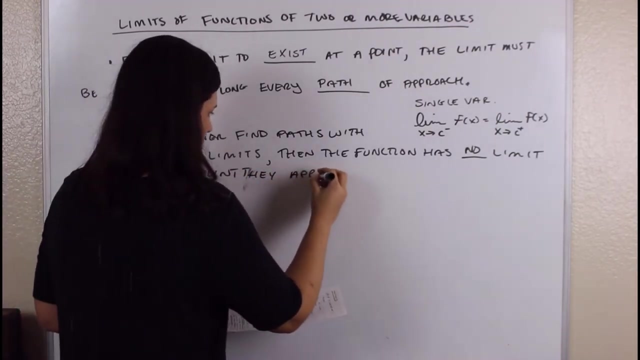 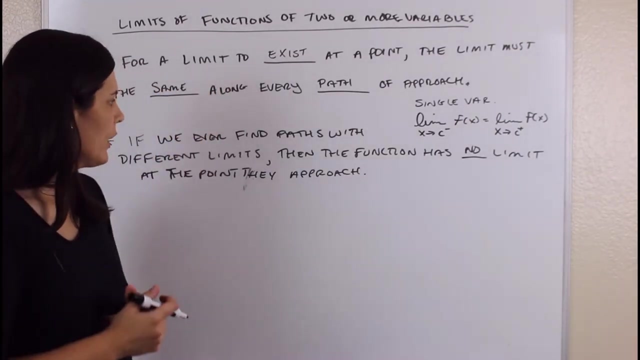 Function has no limit at the point they approach Okay. Sorry, Get there. Point: they approach Okay. So I'm going to show you an image so you can kind of visually understand what I'm talking about here. You can kind of think of it like a cliff. 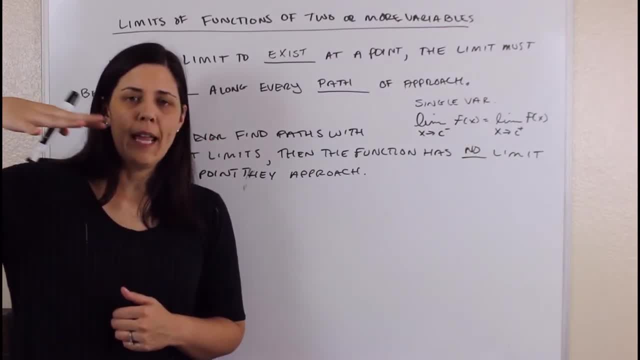 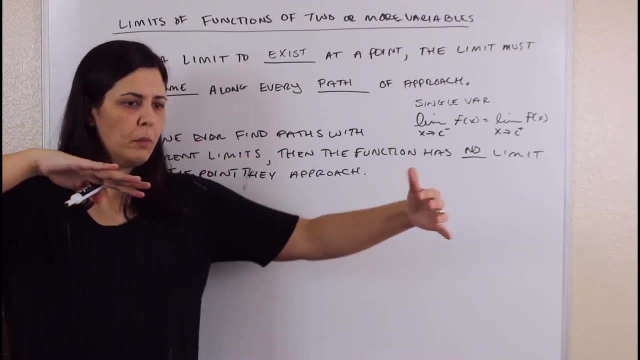 If you could approach a cliff from the land that's at the top of the cliff, that's okay, But to get to the edge, that's the only way there, And then, on the other bottom of the cliff, you are approaching whatever's underneath. 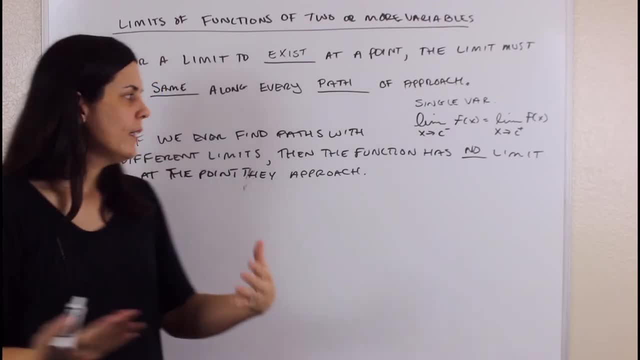 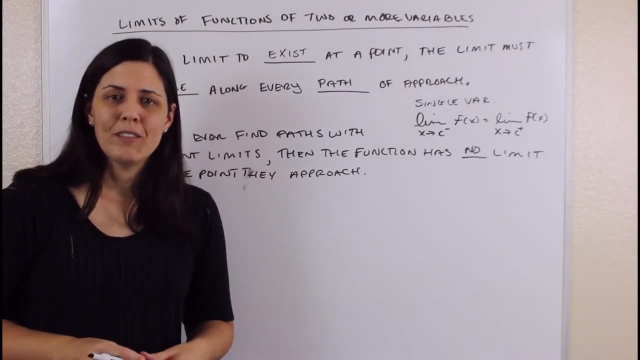 it, And so you would actually be approaching two different values And so that limit wouldn't exist. We would say: no limit exists at that point they're approaching. So let me show you so you can see what I'm talking about. Okay, so here's an example of a function where we would have, like, two different paths of 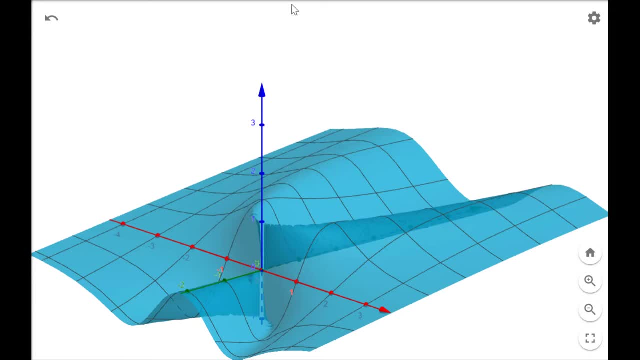 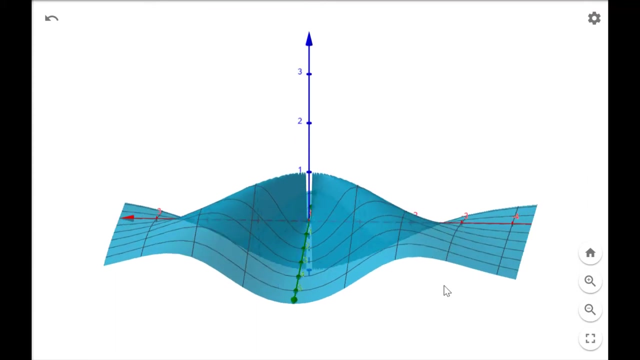 approach and the limit not exist because of what happens. So, for example, consider approaching the origin, which is right down here, zero, zero and along different paths of this surface. So let's say I was approaching, trying to get to zero, zero. 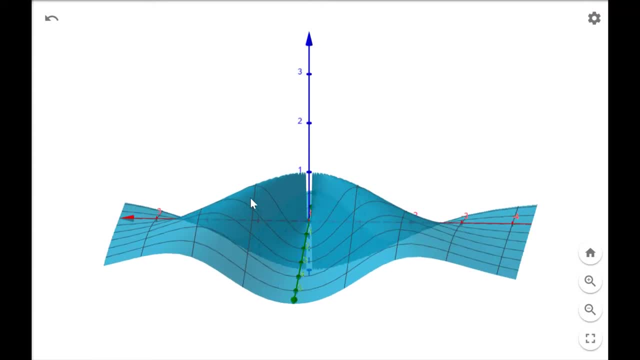 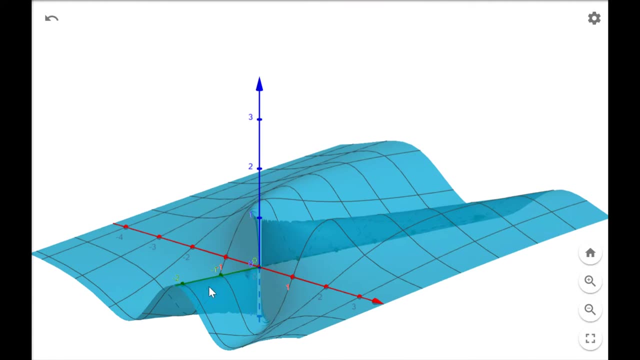 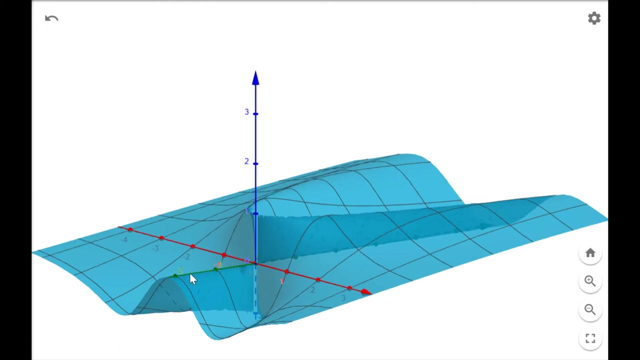 I'm over here. If you kind of notice, this side of this function is going up like this toward one. if I kind of scroll down over here this part right here, if you can tell, approaching the origin. if I walked along here I'd just be already on this axis and approaching zero, zero. 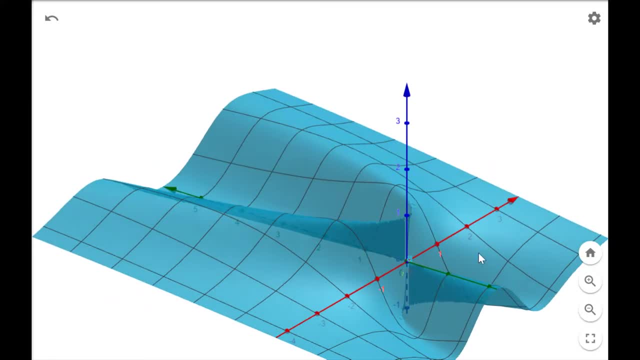 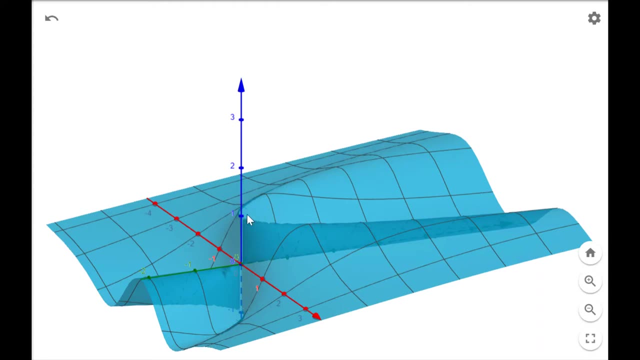 And so different things are happening here as far as how we would end up approaching zero, zero And that whole idea of like maybe the cliff, Okay To where, coming from one side, you're approaching one value, coming from another side, you're. 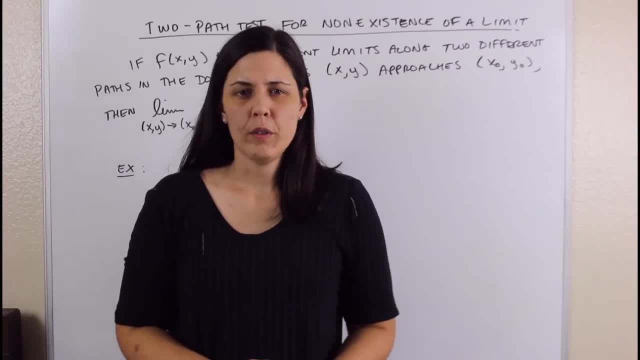 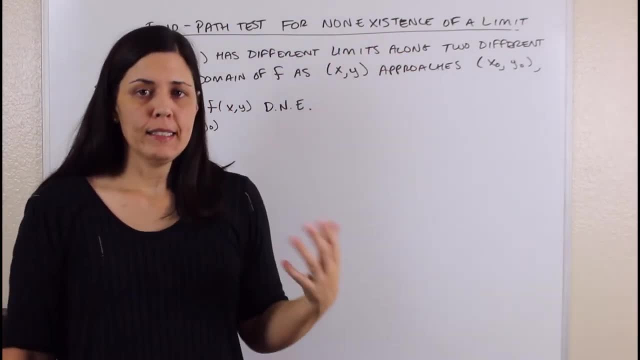 approaching another value. All right, So we have what's called the two path test for non-existence of a limit, And this is a test to let us know if the limit does not exist. Let me read it to you. It's really straightforward. 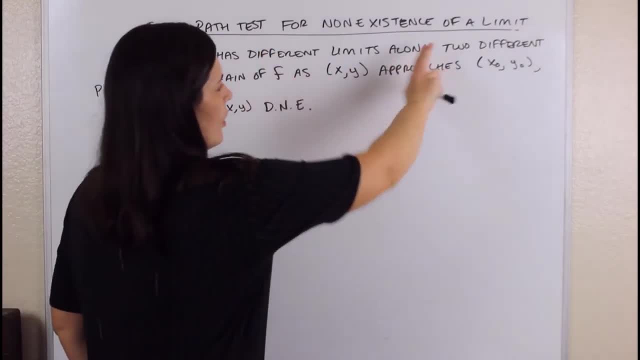 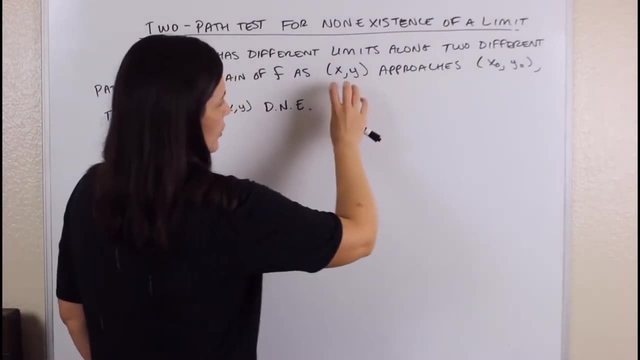 It just says that if your function has different limits along two different paths within our domain of our function, As you're approaching the point you were looking for, So as X, Y approaches X, not Y not, then the limit doesn't exist. 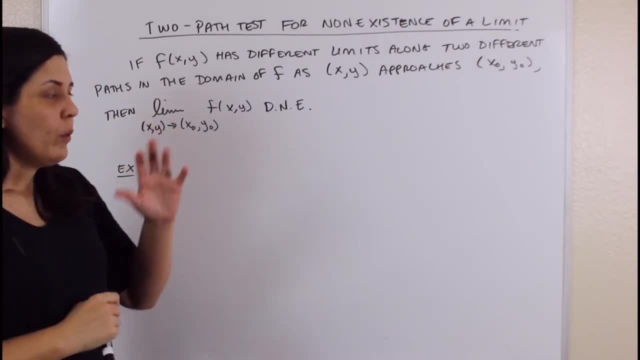 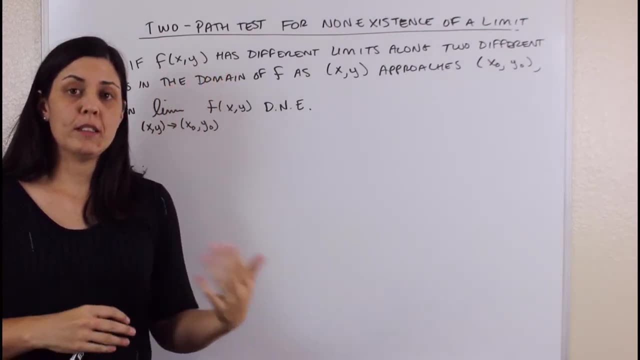 Okay, This is what we were saying. So what I want you to just kind of be aware of what this is not saying. this is not a test for does the limit exist? It's a test to prove that the limit does not exist. 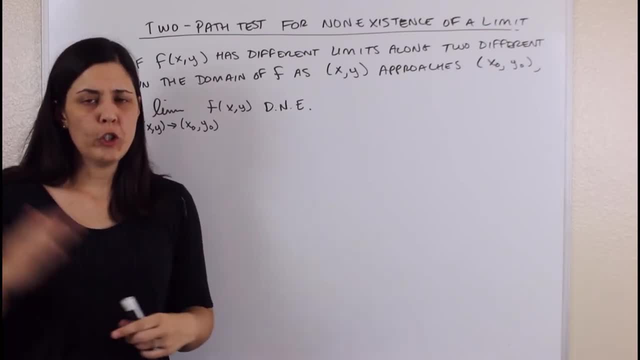 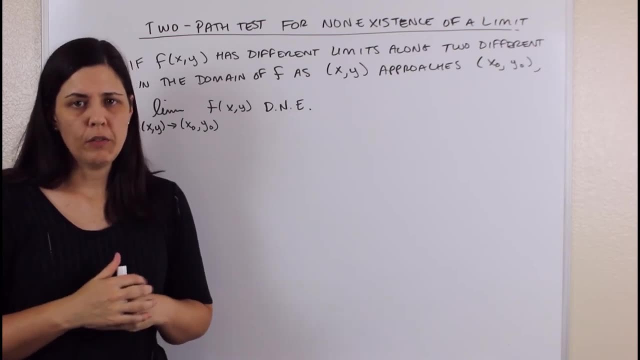 And also what it's not saying is, if you only think about straight line paths, that's not necessarily going to imply that the limit exists, So you have to consider different types of paths, like maybe curved paths as well. So let's try an example. 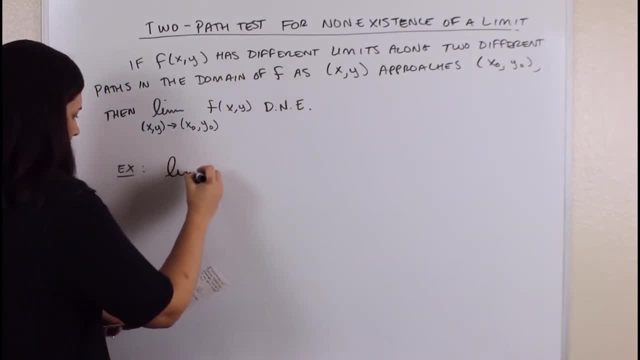 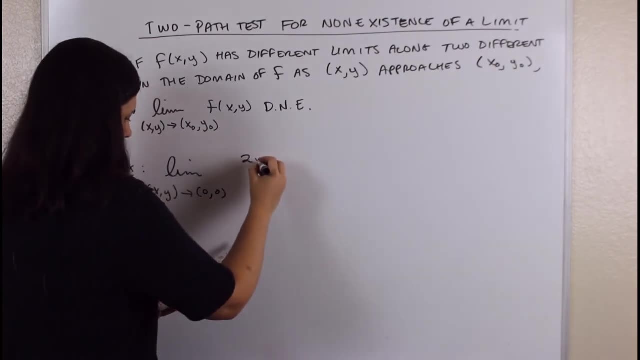 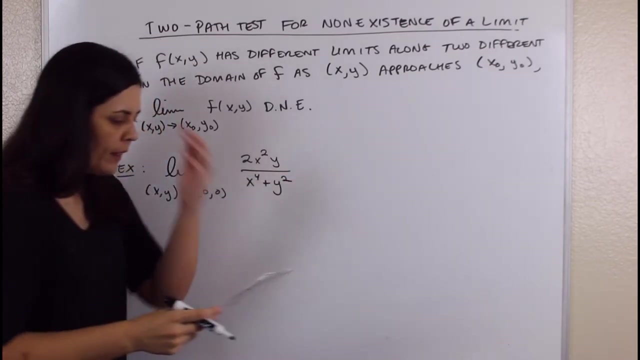 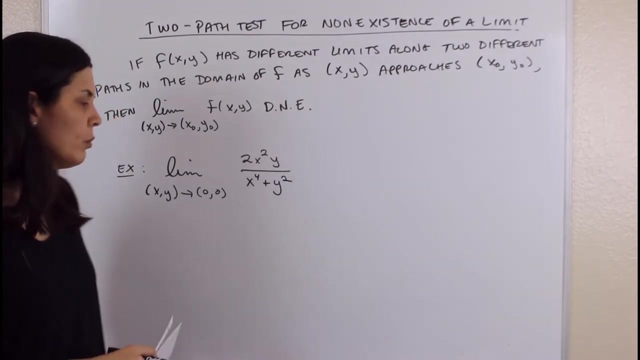 And so we have the following limit: The limit as X- Y approaches zero, zero of two: X squared, Y over X to the fourth, plus Y squared Okay. So what I want to know is: does this limit exist? And If I plug in zero, zero, what's going to be undefined? 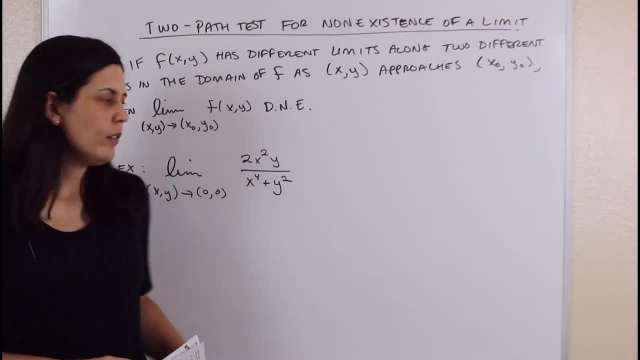 I can try to factor and do different things to see if what I can figure out here, this actually doesn't factor nicely at all with real numbers. So what I'm going to try is to prove that this limit doesn't exist. I'm going to see if I can find two paths. 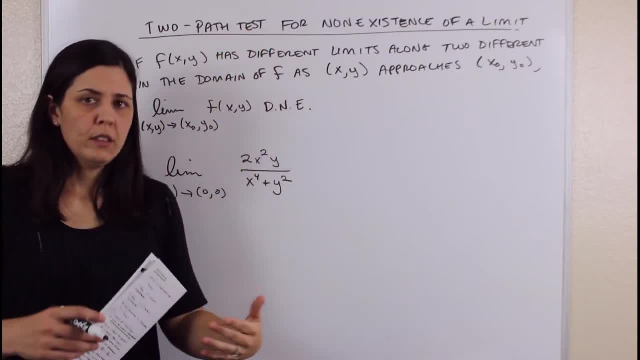 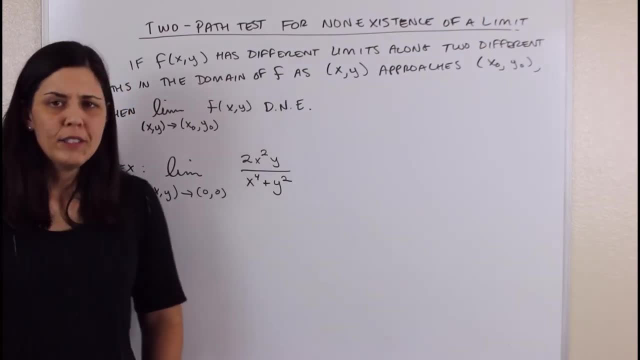 So, for my test, two paths that when I approach two different ways to zero, zero I get different values, Therefore saying the limit doesn't exist, All right. So the paths that I'm going to consider, um, sometimes you have to sort of think about. 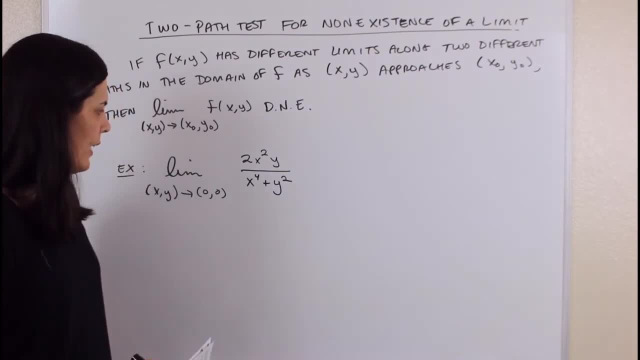 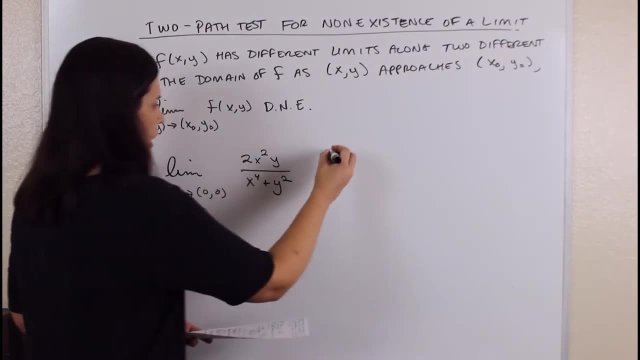 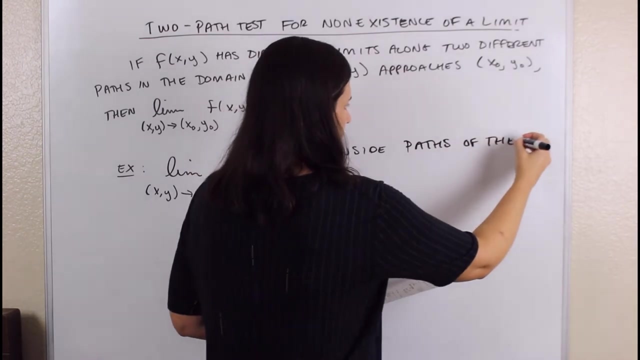 what would be a good path to try, and I'll show you what I mean. It has to do with how the function looks and, when you pick this type of path, how it will simplify. And so here's what I'm saying. I want us to consider paths of the form: Y equals M, X, squared. 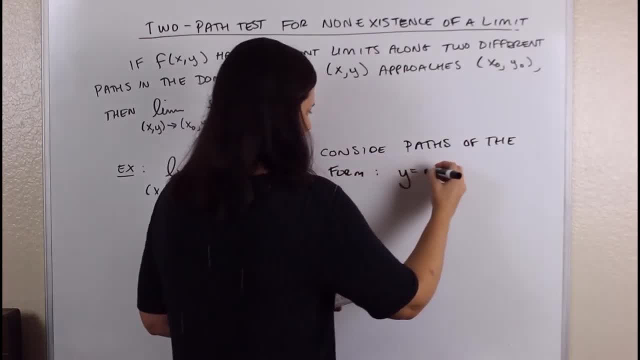 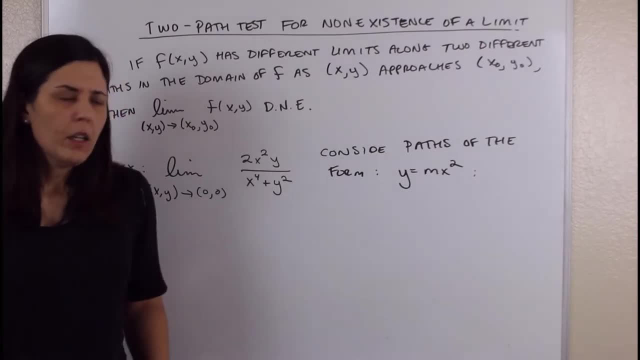 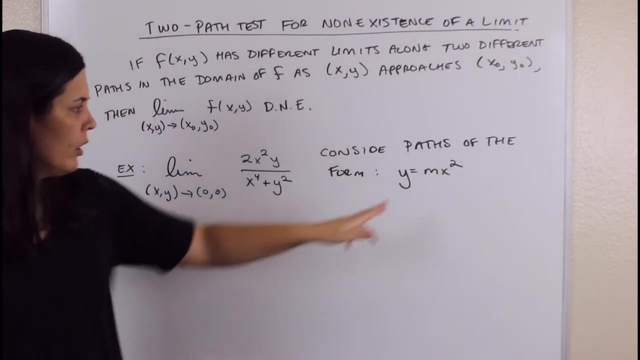 Okay, So, So, So, So, So, So, So, All right, So these are paths that look parabolic, right? This is an X squared equals Y, So it's some kind of parabola With a coefficient that can make it like wider or more narrow. 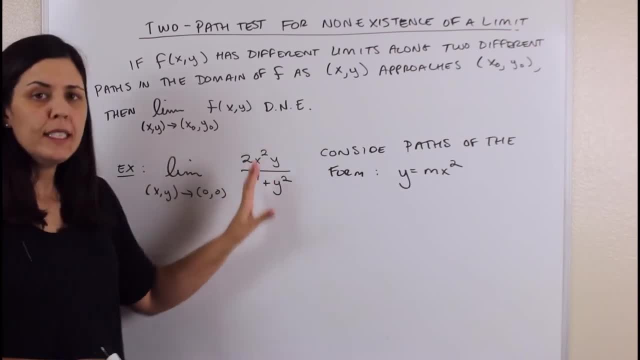 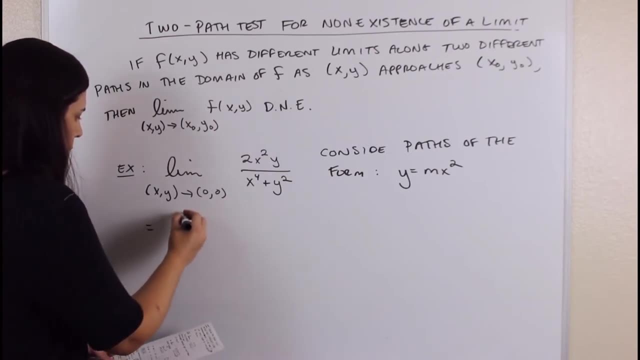 So I want to pick paths of this form, And I kind of had to analyze this to know that this was a good choice, because watch what happens when we do so. we're going to adjust here Our limit, So the limit as X. 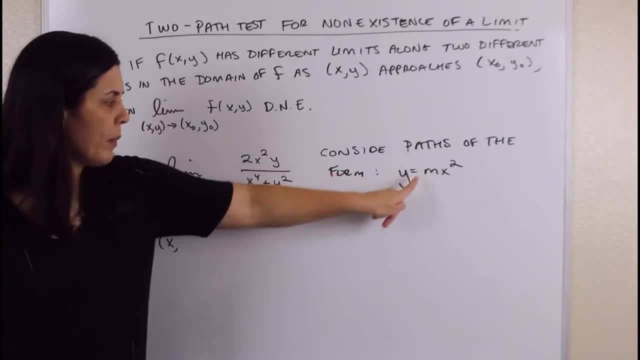 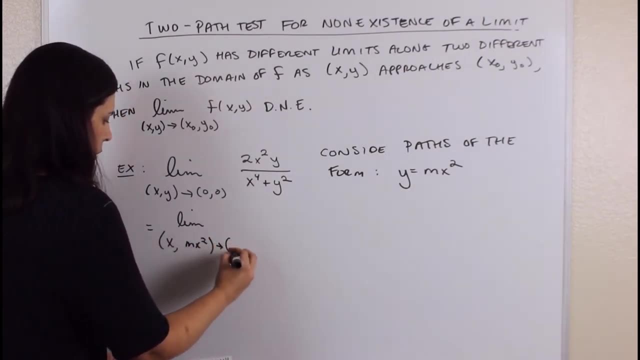 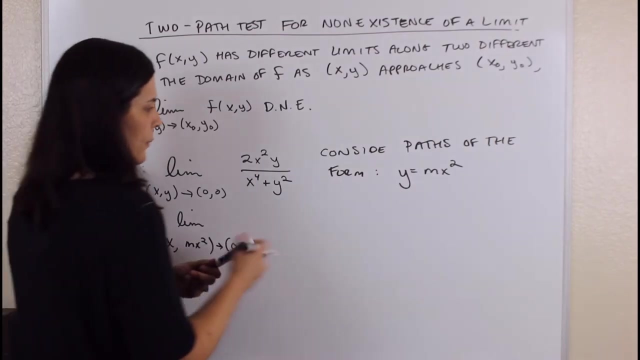 x comma. we are now saying that our paths for y look like mx squared, so x comma. mx squared approaches zero comma. you have to actually do the work over here to think about what this is. it's still zero, but let me just show you why. 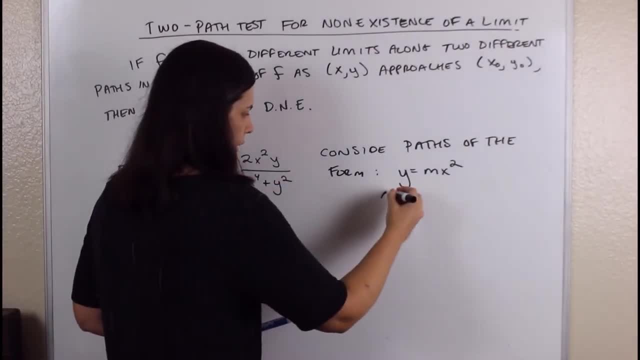 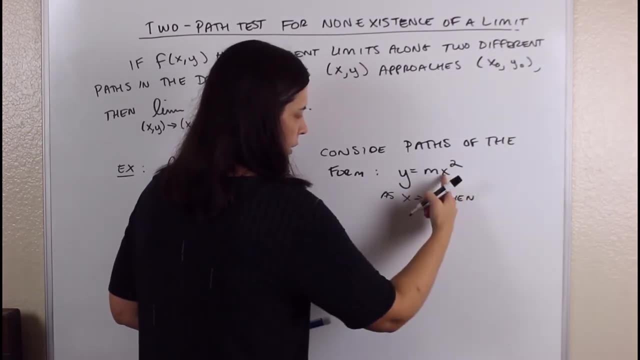 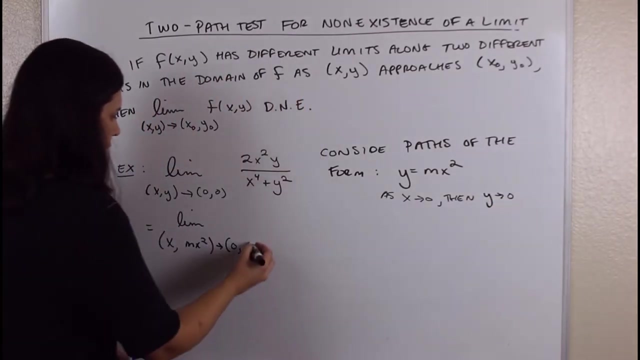 So, as x approached zero, as x approached zero, what does that say here? Then plug in zero. here: m times zero squared y is approaching zero. So this is still approaching zero. okay, but just showing you that you have to actually. 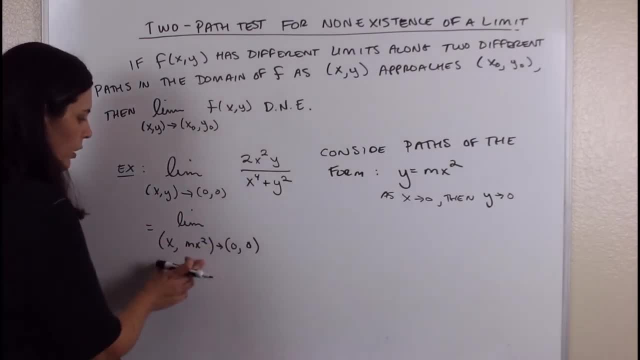 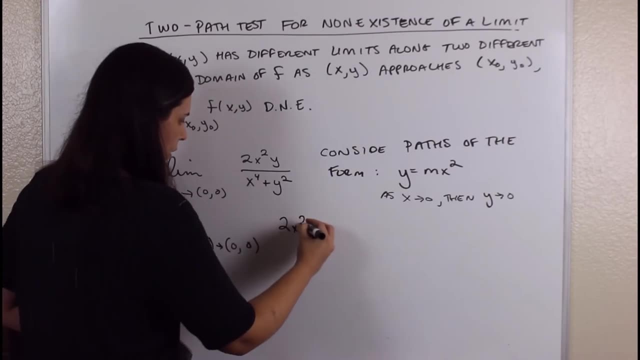 kind of think about that for a second. Alright, so that's this part, changing our terms, of our points. Now let's modify our function 2x squared, and where there's y's, I am replacing it with mx squared. 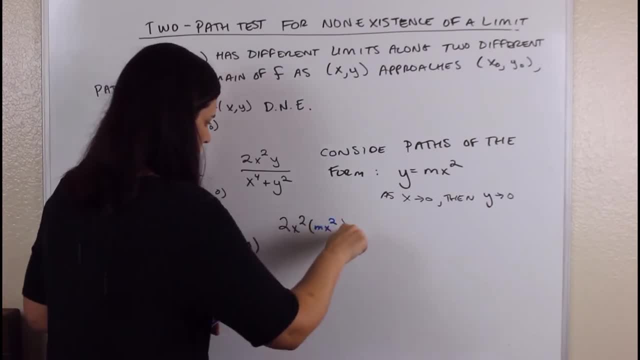 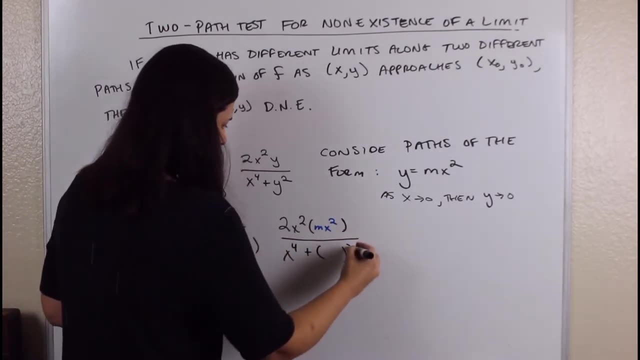 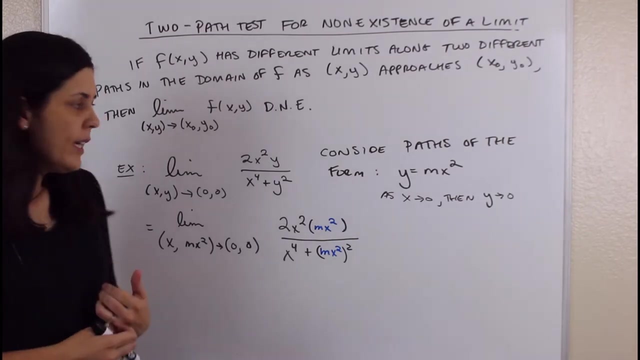 So times mx squared. Okay, That's the numerator On bottom. we have x to the fourth plus y, which is mx squared, quantity squared. Let's simplify and then that way you can see where I'm going with this. So my limit. I'm just going to leave off these points for a second. 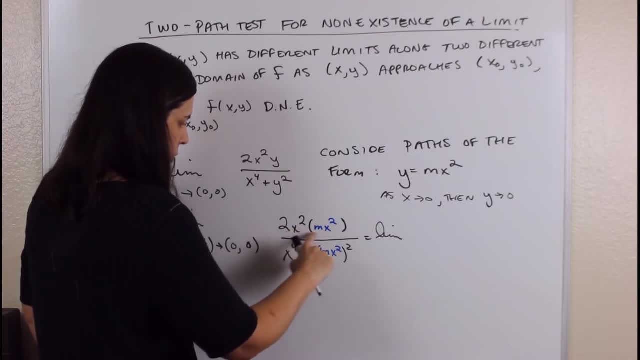 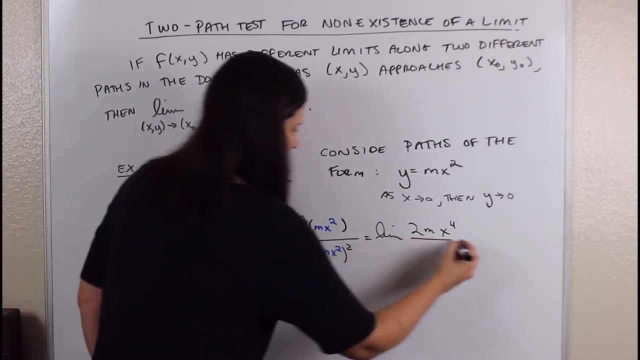 My limit on top- let's see my function becomes. this is 2 times m: x to the fourth, and then on bottom, this is going to be- let's just write it out- x to the fourth. still, but this: 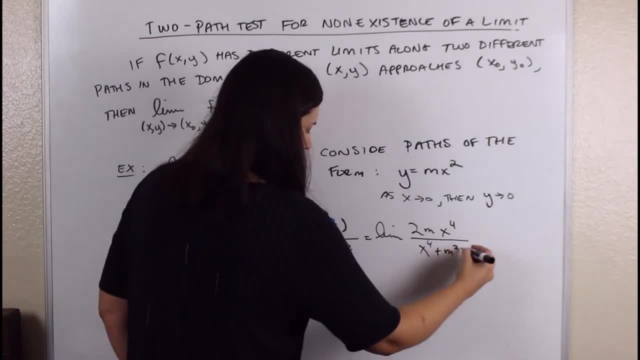 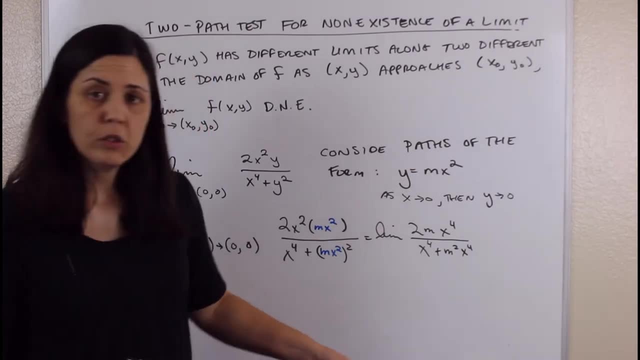 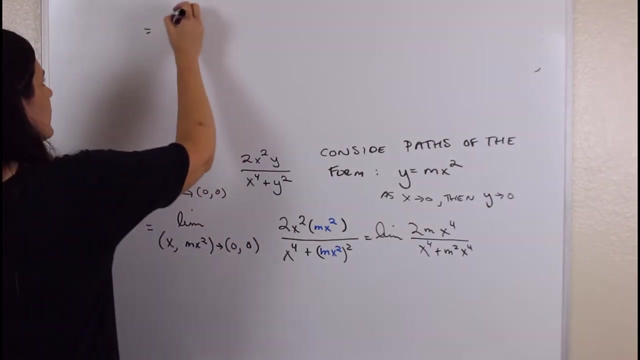 is m squared x to the fourth, m squared x to the fourth, And then we can simplify some things. Notice, all the terms have an x to the fourth in it, so let's go ahead and simplify that. So we have that, this limit on top 2m, because we're going to divide out that x to the fourth. 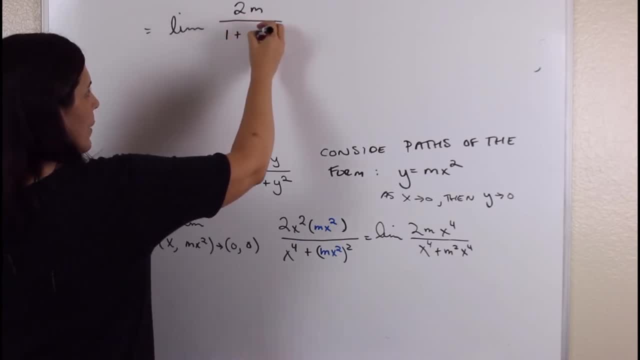 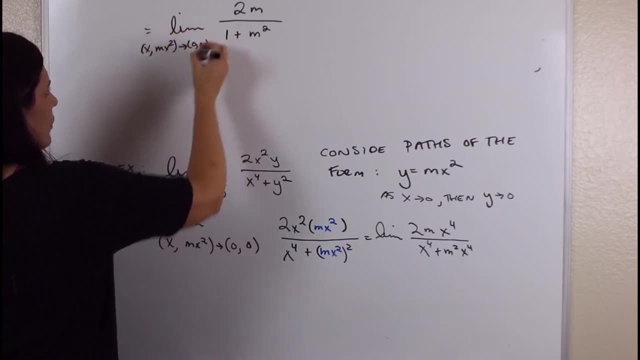 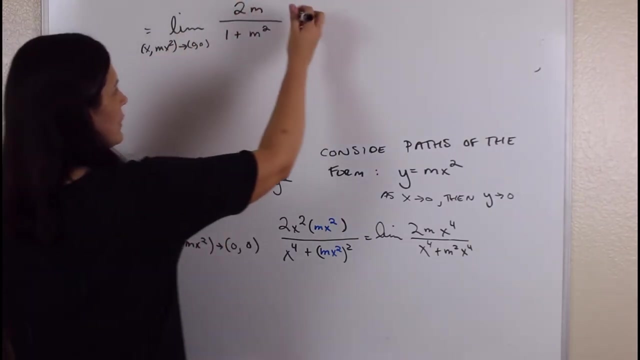 here, here and here, over 1 plus m squared, And this was as x comma. mx squared approaches 0, 0.. Okay, So what does this say? Notice that there's no more x's left, so this actually just equals this. 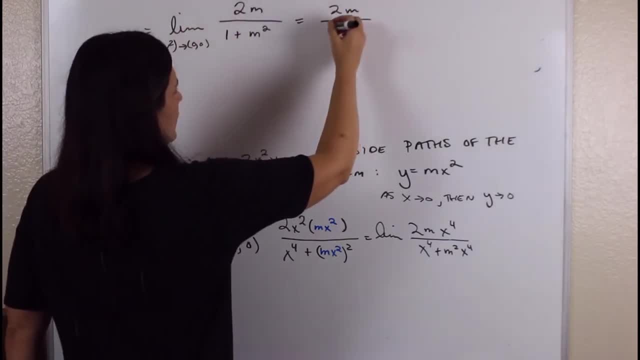 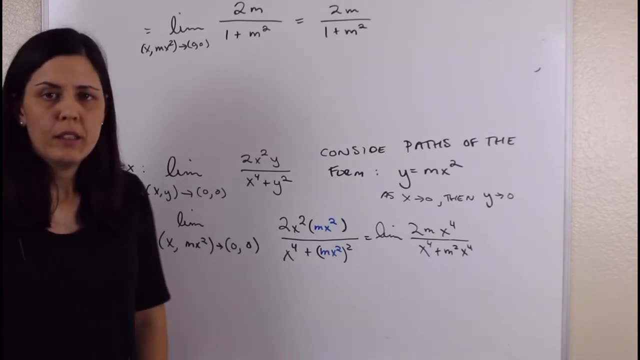 If we try to plug in 0 for x, there's no x's remaining. So this is 2m over 1 plus m squared, And so you have to sort of just say: well, what does this mean? This is my limit, this is l, this should be l, but consider two specific paths. 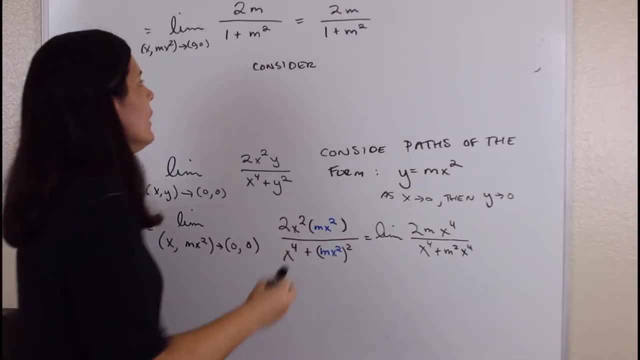 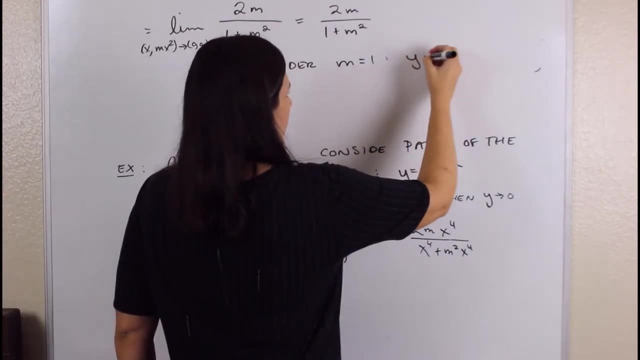 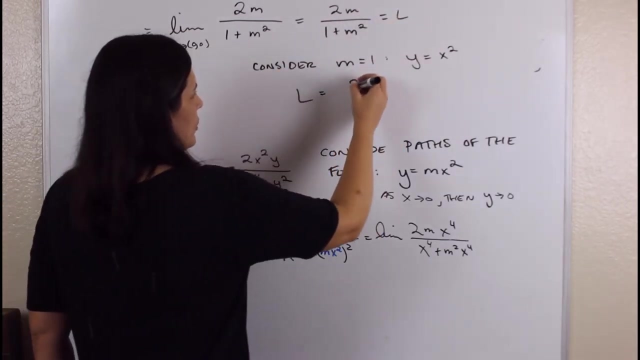 Right now, I kind of generalized it- any parabolic path like this. So what if I say I want the path when m is 1?? So when y equals 1 times x squared? okay, So then my limit here l. let's just write that there l would be 2 times 1 over 1 plus. 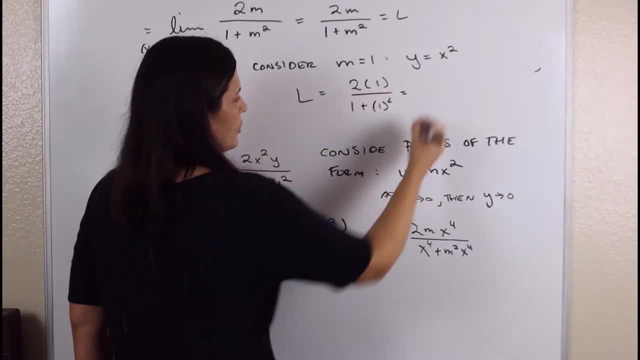 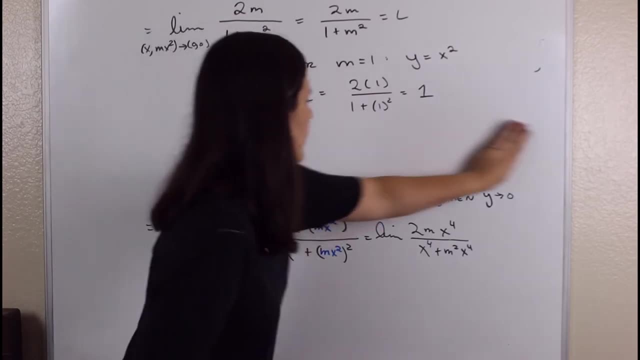 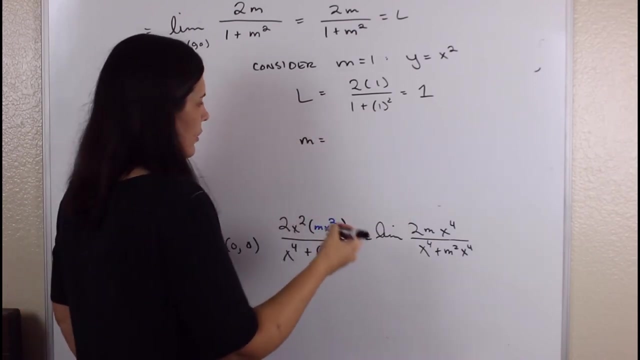 1 squared. Okay, So that's 2 over 2.. So that's 1.. All right, Well, let's say I choose m to be a different number. Let's say, let's just go right here. Let's say m is negative 1, or 2, or anything else. 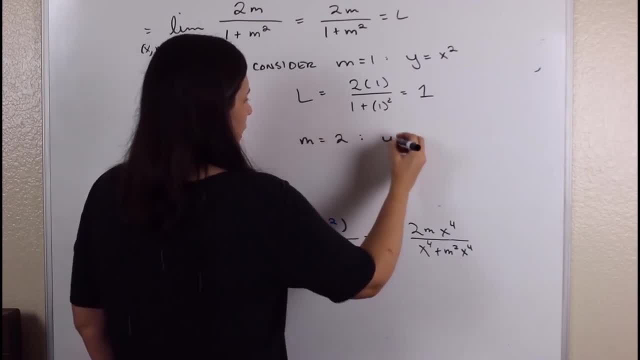 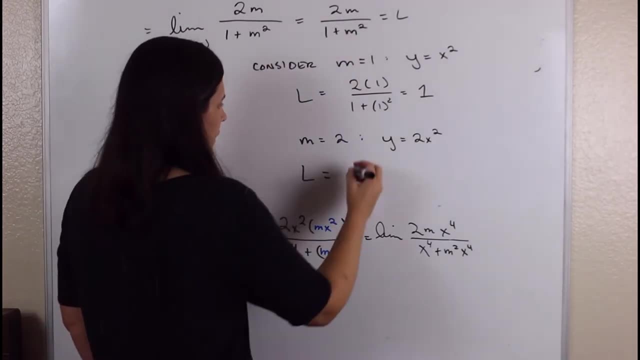 So I'm going to go with 2.. So then y is 2x squared. So then my limit value. what I'm thinking is my limit is 2 times 2 over 1 plus 1 squared. Okay, So that's 2 over 1 plus 2 squared. 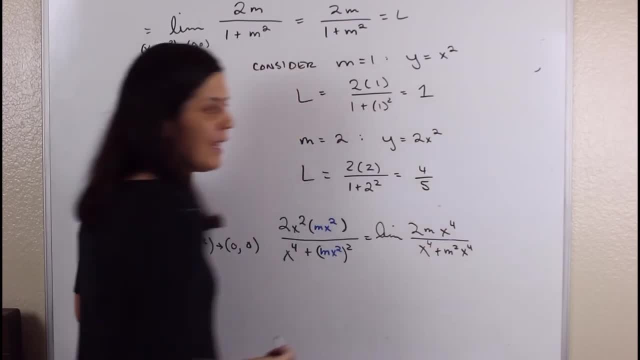 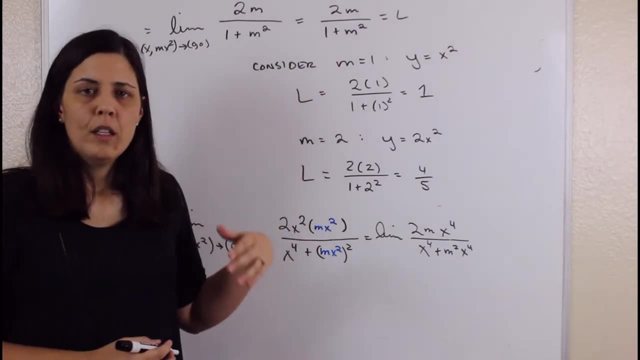 So that's 4 over 5. And they're different. okay, And let's say you pick two numbers for m and you got the same value. you might want to just try a third one and see if you get a different value, to see if you can just find. 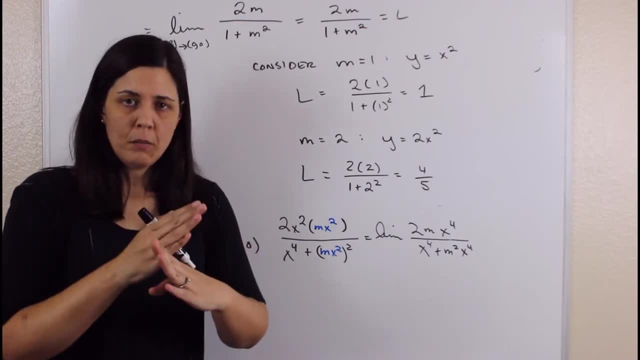 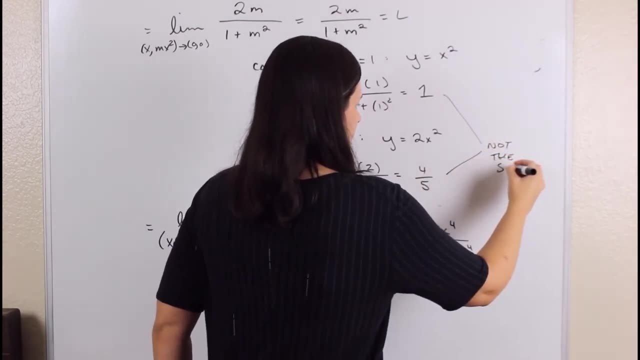 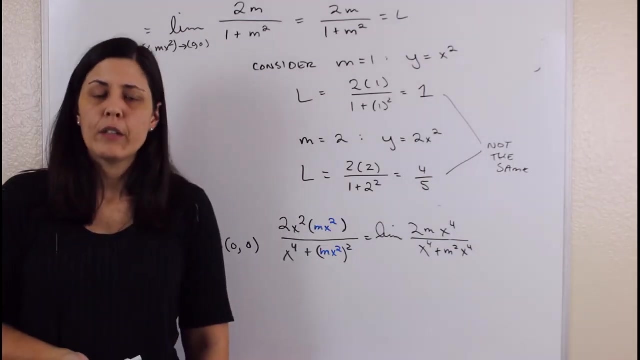 two, two paths where the limits don't meet the same thing, don't equal the same thing. so then this limit doesn't exist. Because these are not the same, this limit doesn't exist. Okay, This limit doesn't exist. We just took two different paths, tried to approach 0, 0, and got different values. so 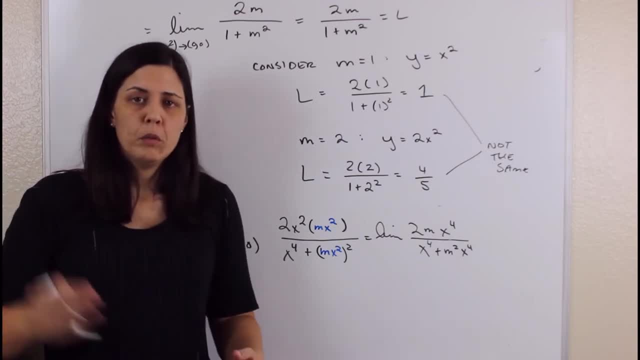 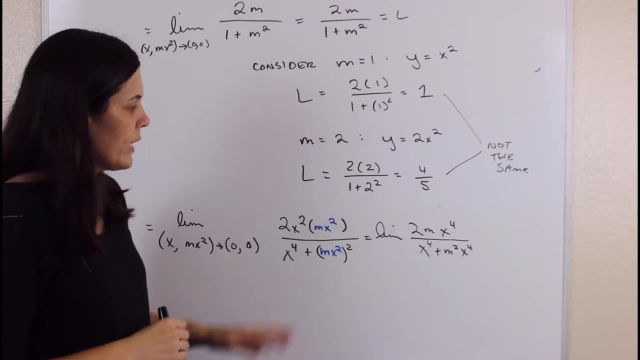 therefore it doesn't exist. Think about it in single variables. if you came in from the left and the right, you're getting two different values as you approach this same singular point. So you can say by the two-path test, this limit doesn't exist. 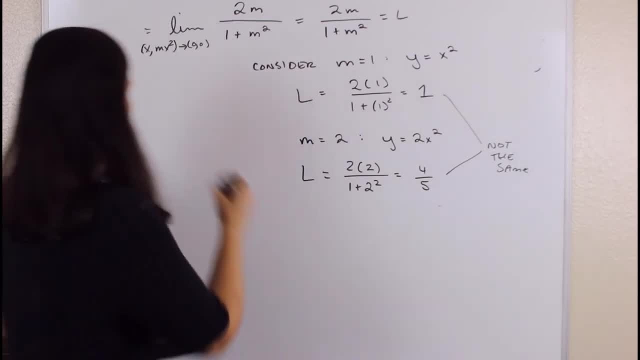 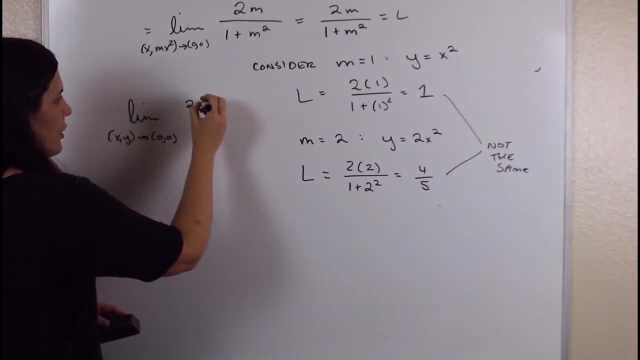 So let's just put that there to be formal. So this limit as x, y, z, Okay, As x y- approaches 0, 0 of our original function, which I think was 2x squared y over x to the. 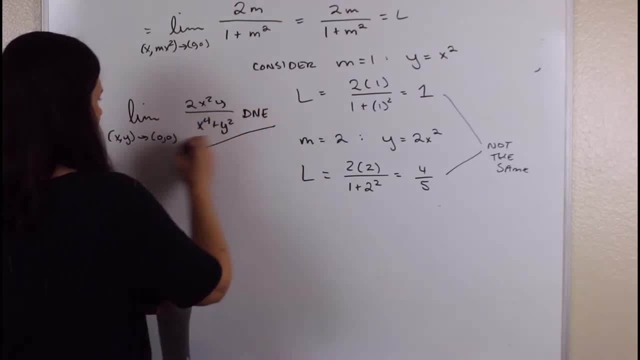 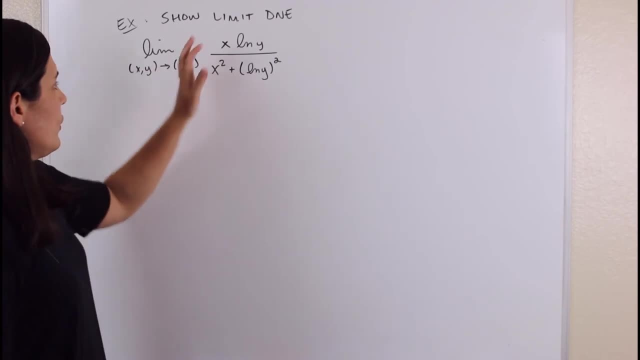 fourth plus y to the second does not exist by the two-path test. Okay, let's try another one. So we're going to show that this limit doesn't exist as we approach the point 0, 1, where our function is x times the natural log of y divided by x to the fourth plus y to the. 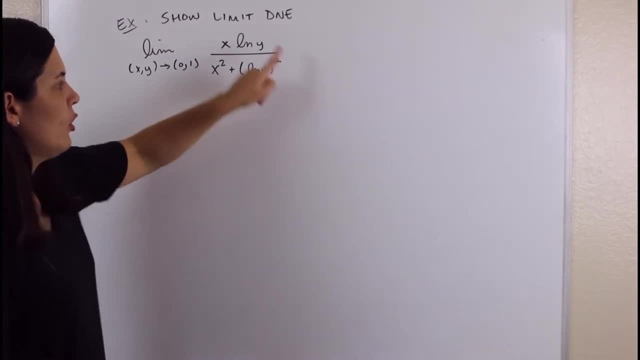 second. So we're going to show that this limit doesn't exist as we approach the point 0, 1, where our function is x times the natural log of y divided by x squared, plus natural log of y quantity squared. So let's think about some paths and we'll try them and see what happens. 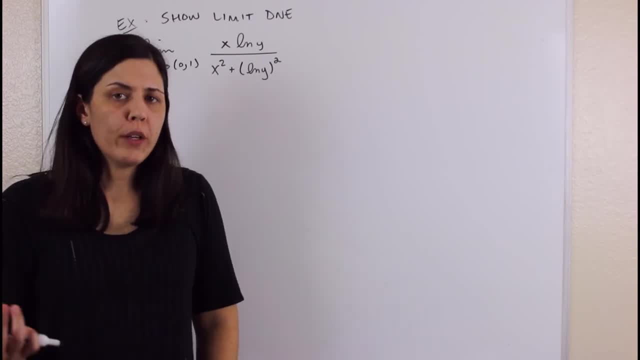 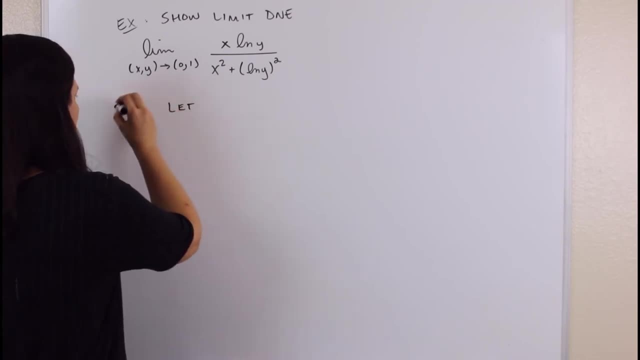 So when we pick a path, we still have to end up approaching the same point that we're supposed to approach, which is 0, 1.. So I'm going to let so for path 1, I'm going to let y equal 1.. 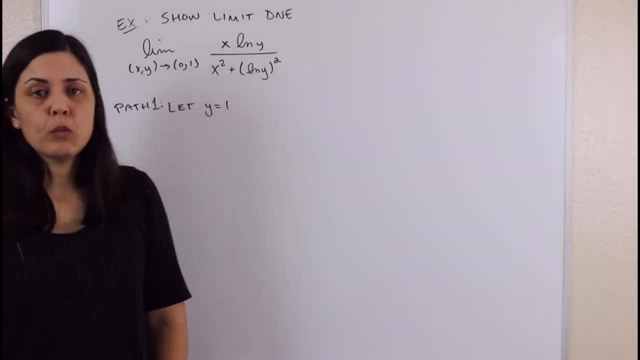 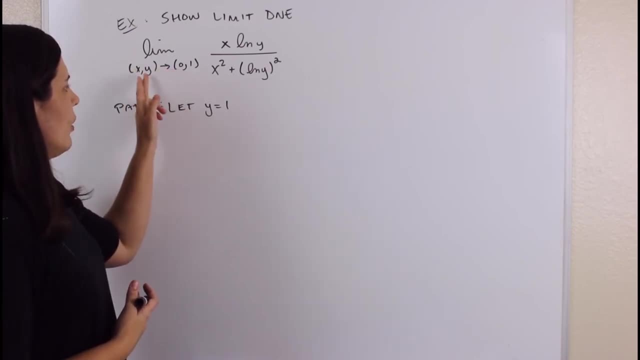 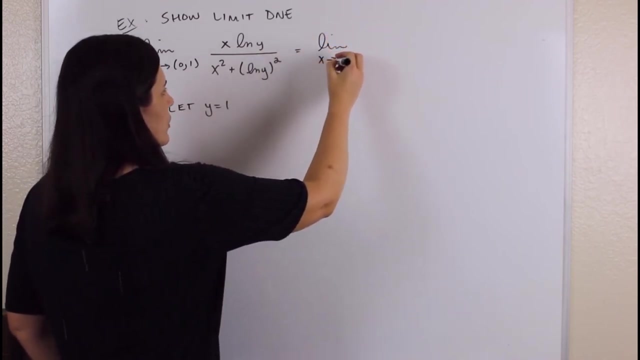 I'm going to pick a straight line path where it's line y equals 1.. Okay, Think about it. That still approaches the same point, because x approaches 0 and then if y is 1, it's definitely approaching 1.. So, if I go right into my limit here, this is now the limit, as x goes to 0, since y is. 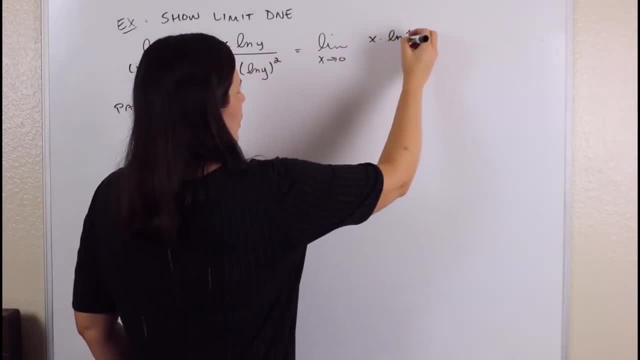 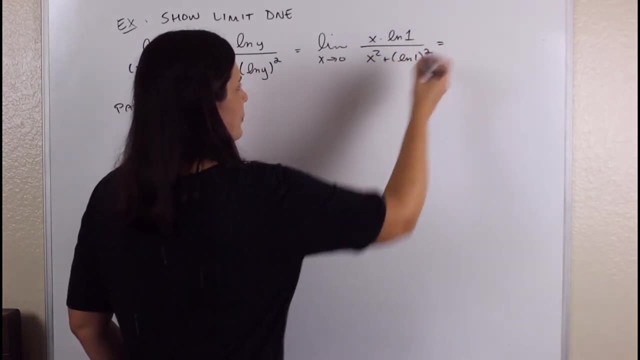 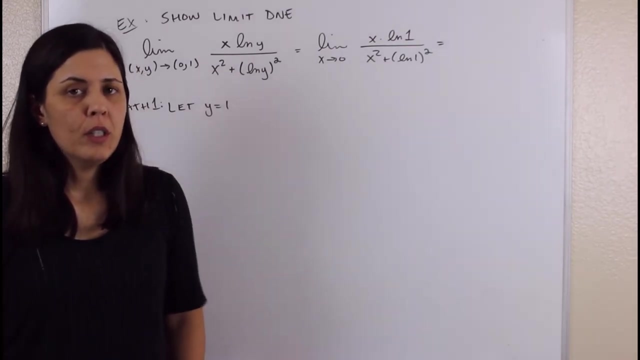 1.. And then x times natural log of 1 over x squared, plus natural log of 1 quantity squared. Okay, Now simplify Natural log of 1.. If you remember, That's just 0.. Because natural log is saying e. to what power equals this number? 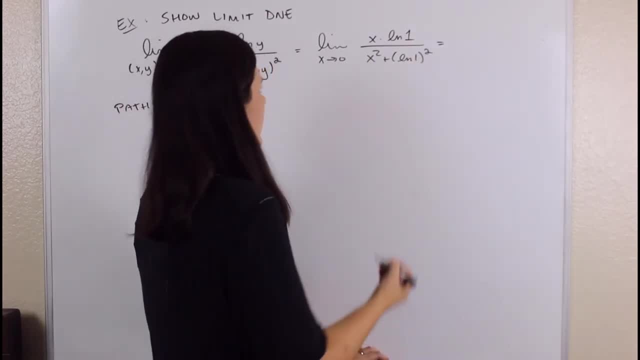 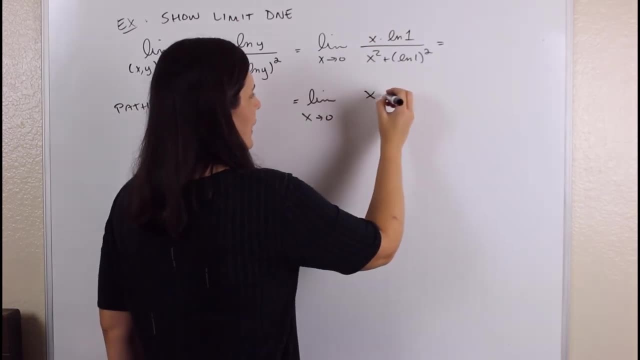 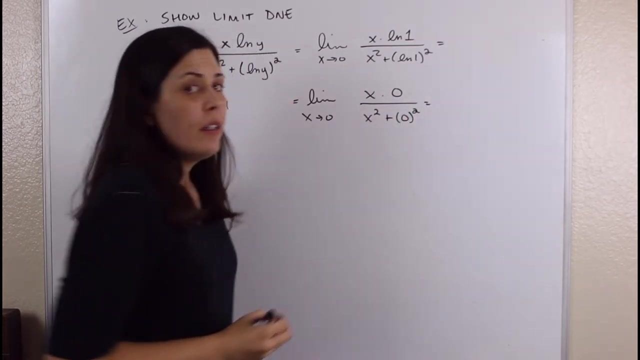 So e to what power is 1?? The answer is 0.. So this is the limit. let's go down here actually The limit as x approaches 0 of x times 0 over x squared plus 0 squared. Now, if I simplify this, my numerator is 0.. 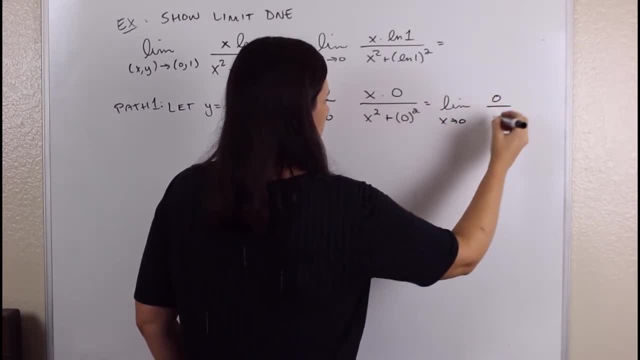 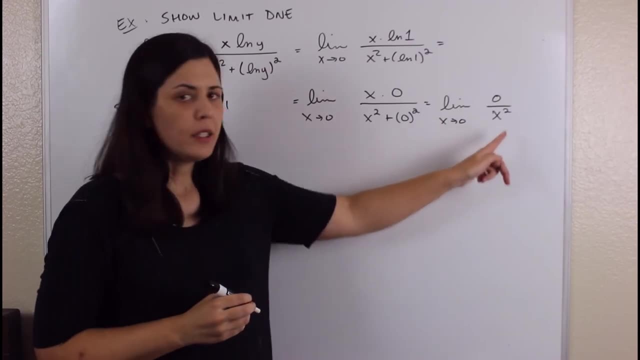 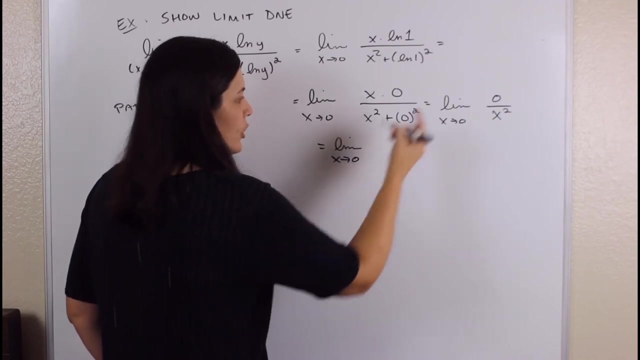 So I have my limit as x goes to 0.. Over my denominator, which is x squared. And now be careful, don't take your limit just yet, because if I plug in 0 for x, it's going to be undefined. But if you think about it without approaching anything, I still actually have to simplify. 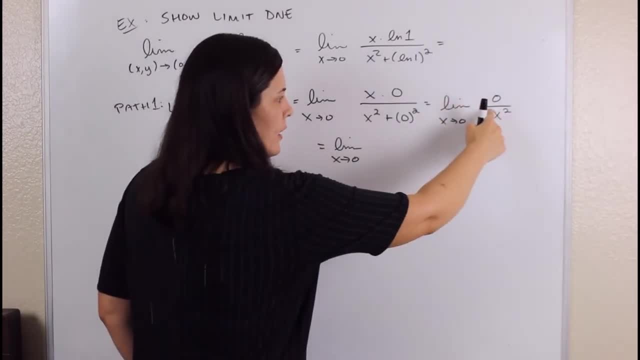 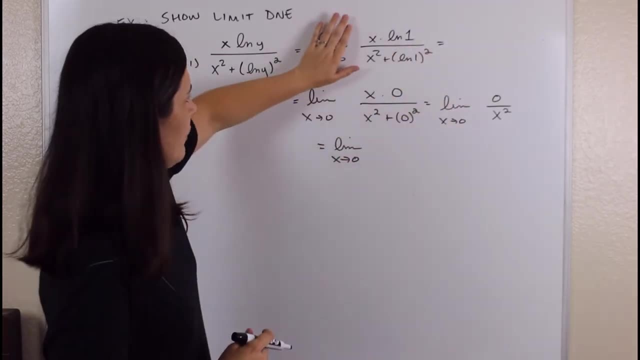 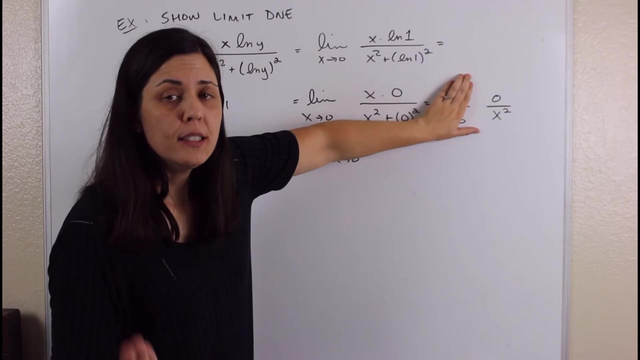 So I'm still on the simplify step: 0 over anything other than 0. So as a function, so if I kind of take off limit from all of these steps, if you just sort of think about simplifying our function, So if I ignore all of this, 0 over x squared is just a constant 0.. 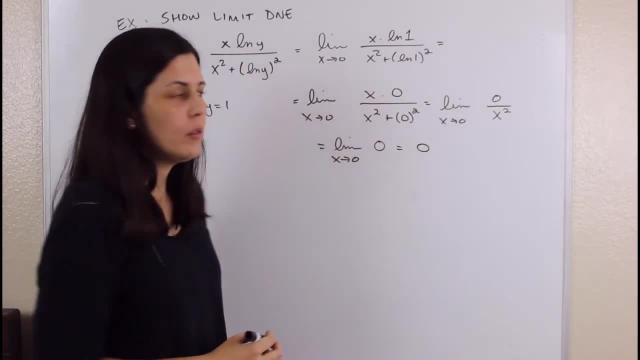 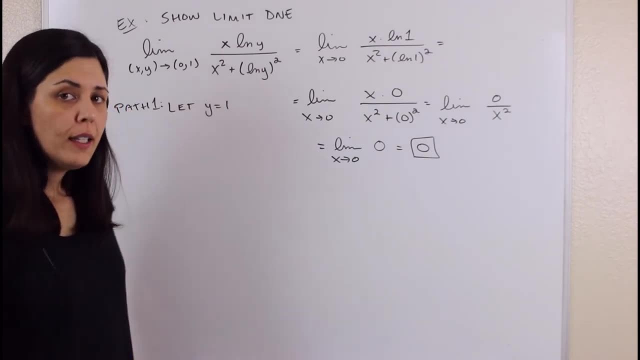 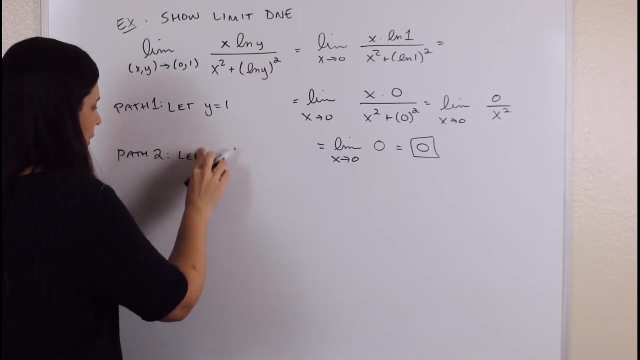 So this is really the limit of 0,, which is 0.. So approaching along the path y equals 1,. our limit value is 0.. Let's try a different path and see what we get. So path 2, and let's see what's a good path. 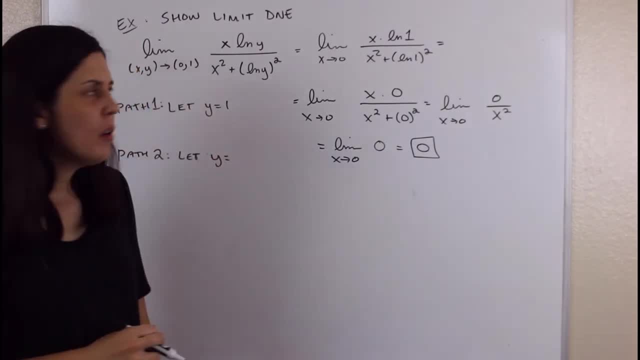 If I sort of think about this, Okay, If I sort of think about the fact that I'm using natural logs, maybe I should introduce e- e to some power, And so what I'm going to do here is I'm going to let my second path be e to the x. 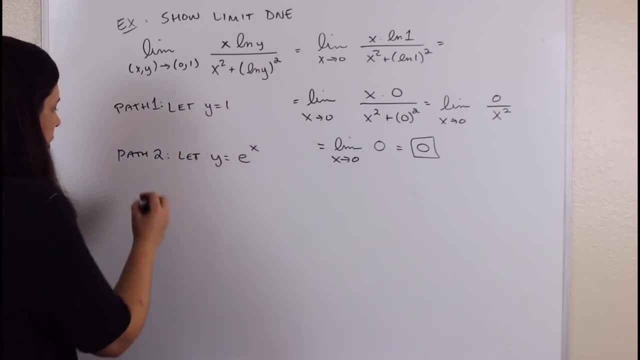 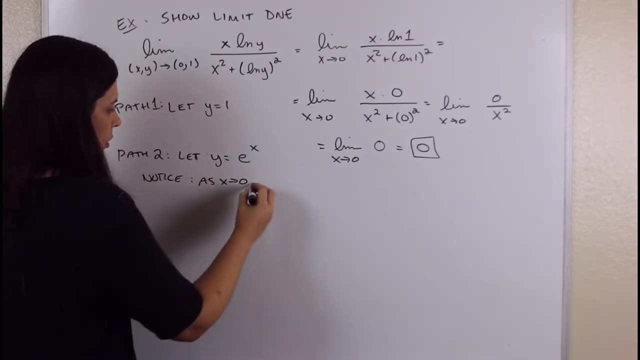 Now we have to just make sure that we're still going to approach the same point. So we'll say: notice, as x approaches 0, then y equals e to the 0 approaches 1.. Okay, So we are still, in fact approaching the same value. 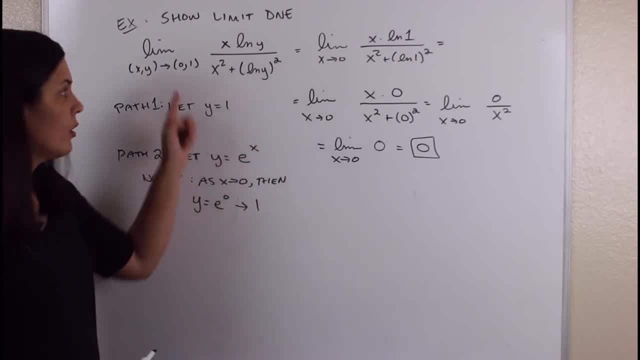 X goes to 0, and if we plug in 0 here, y is going to 1,, which is good, Okay, So let's use that as our path number 2.. So from here plugging that in for y. 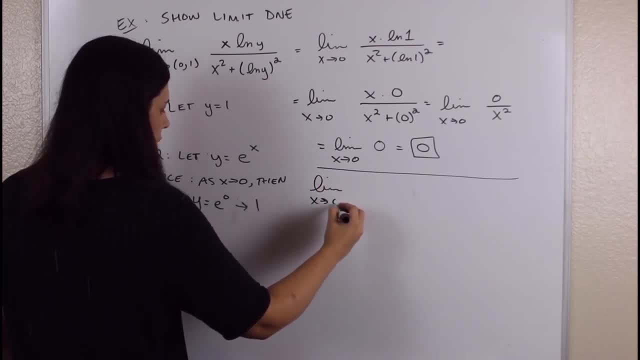 So the limit as x goes to 0, and then y goes to e to the x, We are going to- actually I guess I should put that there- So x and then e to the x, 0, 0.. Okay. 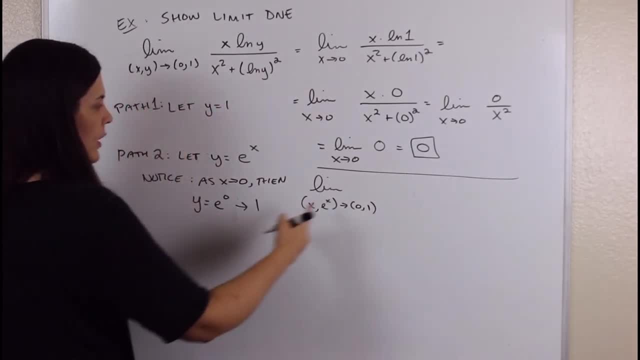 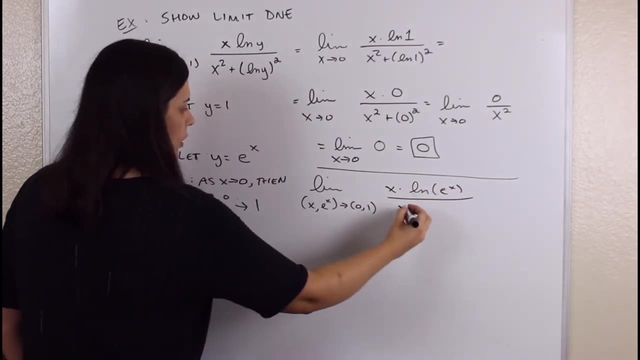 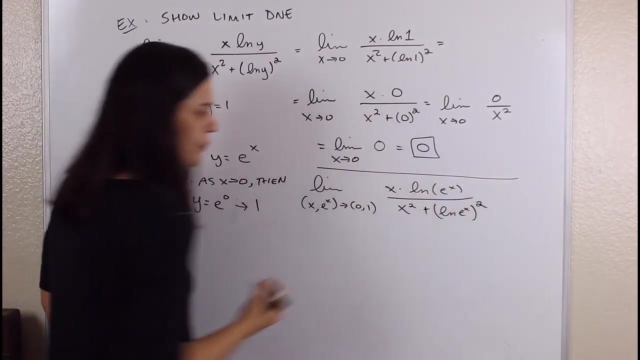 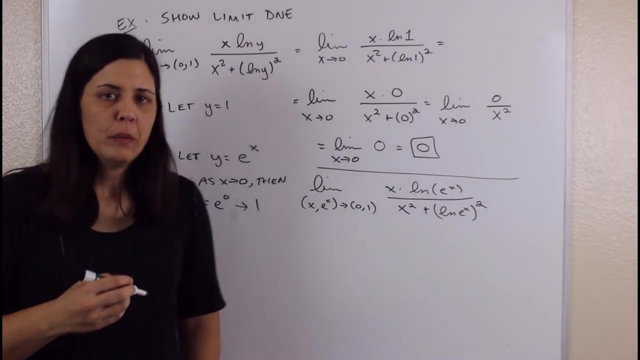 So we have x times natural log of e to the x over x squared, plus natural log of e to the x quantity squared. All right, Now let's simplify. Natural log of e to a power is the power, Because remember what this is asking. again, natural log is saying e to what power does. 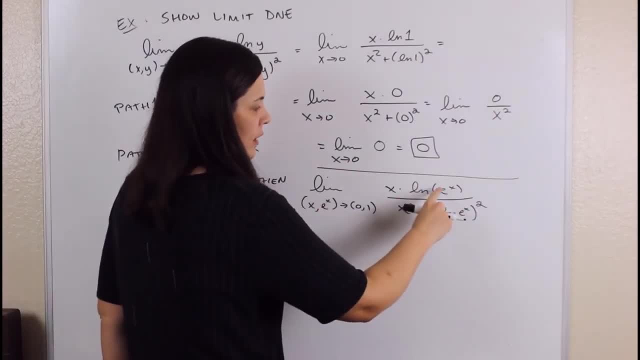 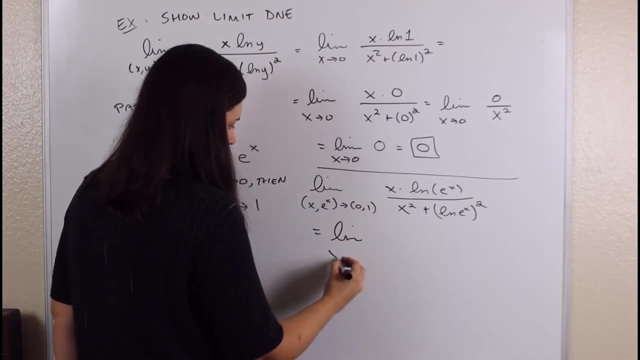 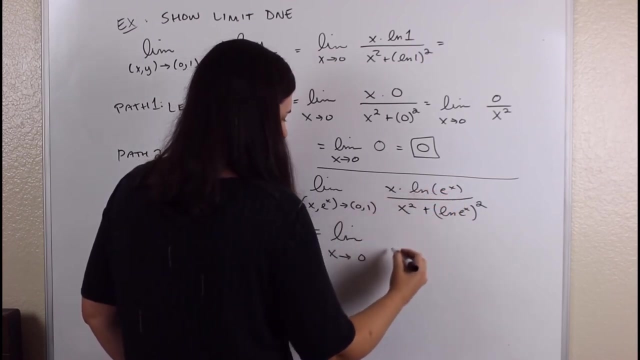 this equal Well natural log of e to the power. the answer is right there, it's x, it's the power. So this is our limit. as x, just focus on x. x goes to 0 on top. This is going to be x times x, because what I've been saying, this whole thing here, is: 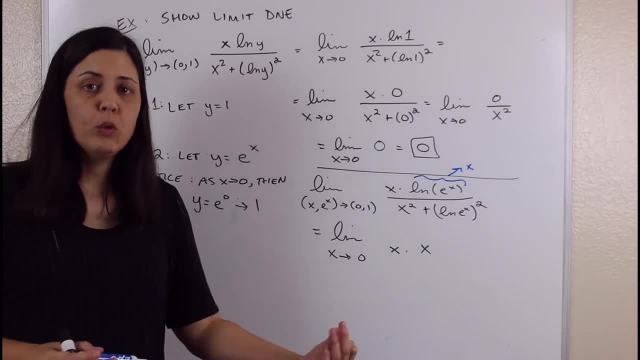 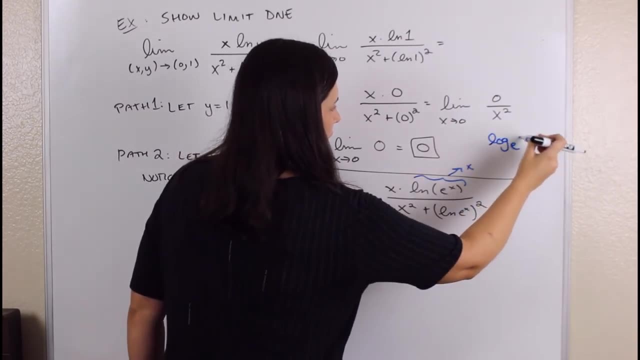 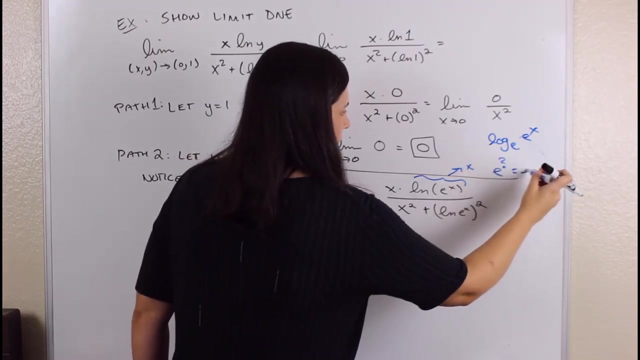 just x. If you go back and think about your rules of x, rules of logarithms, I'll show you. if it, I'll put my fingers on that. This is log base e and this is of e to the x. So it's asking you: e to what power is e to the x? 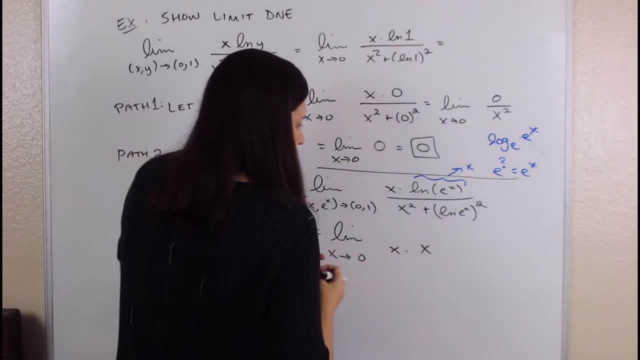 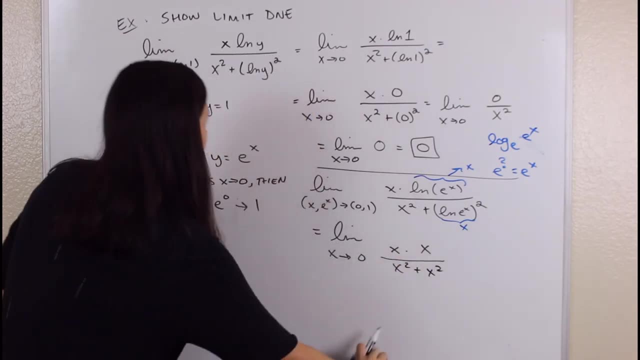 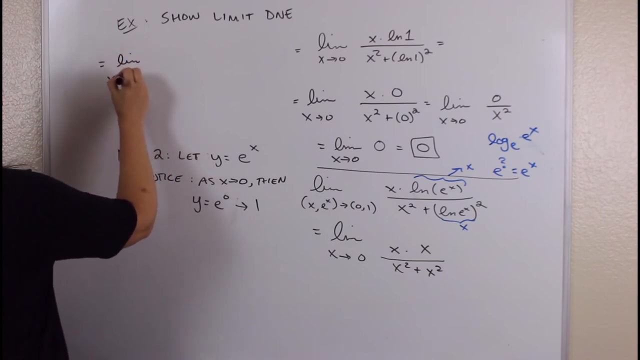 So the answer is that power, And so this is also just x. So this is on bottom x squared plus x squared. So let's move back up here And we have the limit as x goes to 0 on top, x squared on bottom 2 quantity x squared. 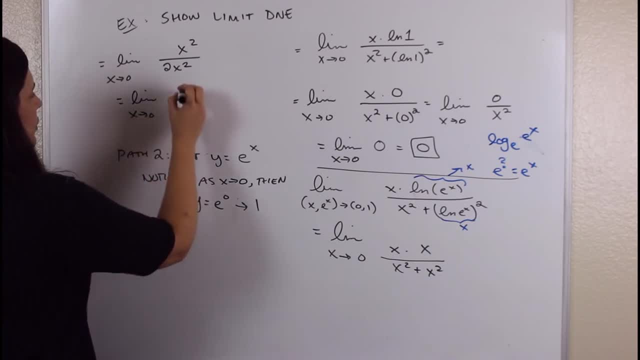 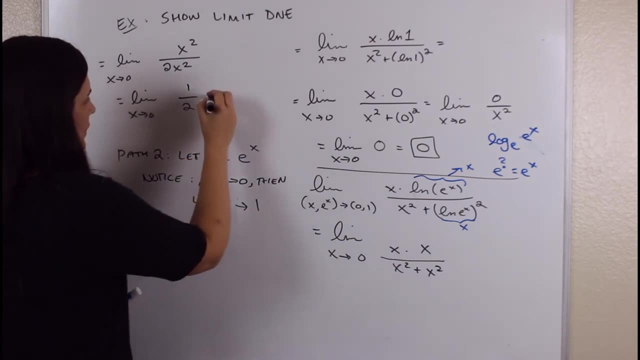 And if we simplify, this is the limit, as x goes to 0, of 1 over 2, because the x squareds divide out And now we consider plugging in 0, but there's no more x's, so this is 1 half. 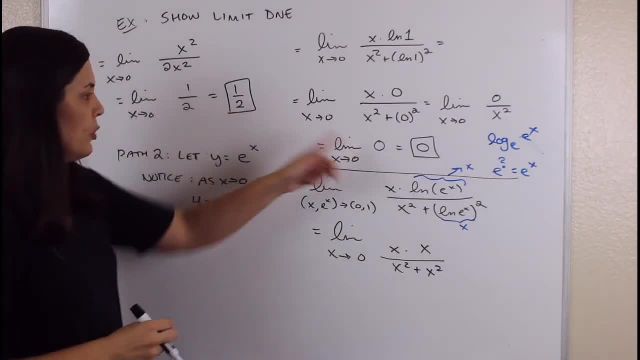 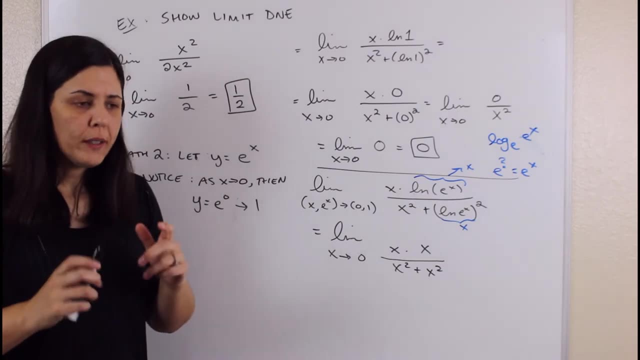 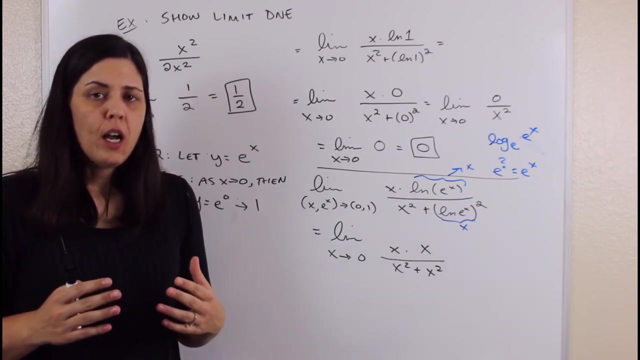 So, by the two-path test, we got two different limits. So you can say, therefore, this limit does not exist. And so, like I mentioned before, real quick, Just because two straight line paths, or even all straight line paths, have the same limit. 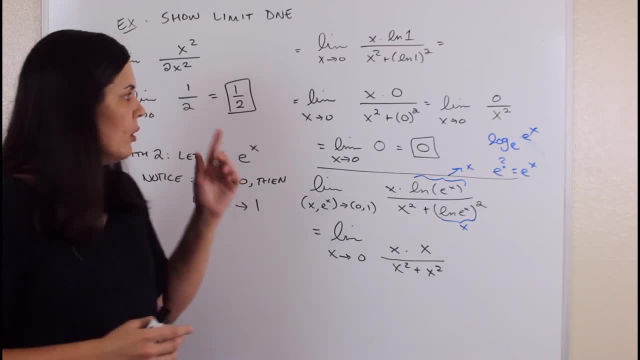 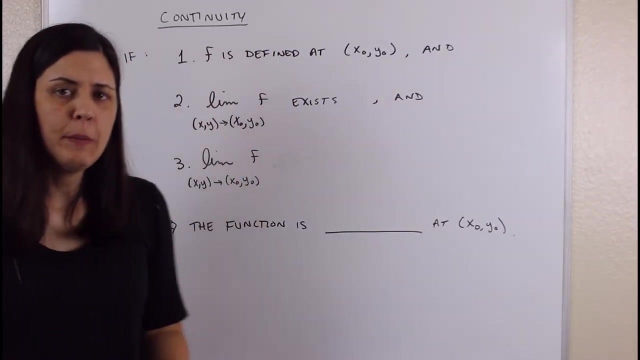 you have to consider curved paths as well. So we did one straight line path but one curved path. So the fact that they didn't equal the same thing was good, All right. So next we're going to talk about continuity. So, for continuity, this idea here is exactly the same as what you know from single variable. 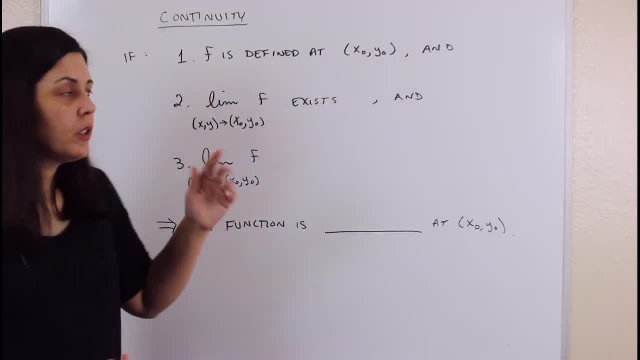 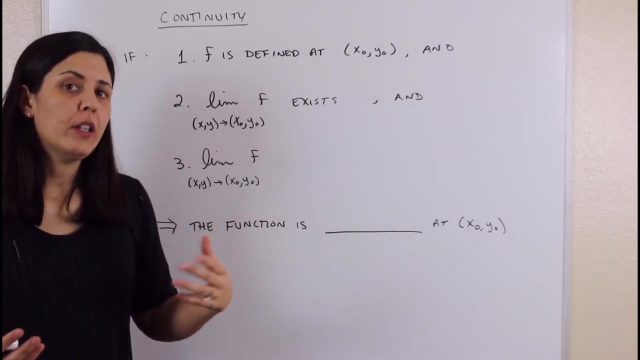 calculus. These three things have to be true. So, number one, your function is defined at the point you're approaching. Number two, the limit of that function exists as you approach that point. And number three: think about it, what either you remember or what you could just sort of. 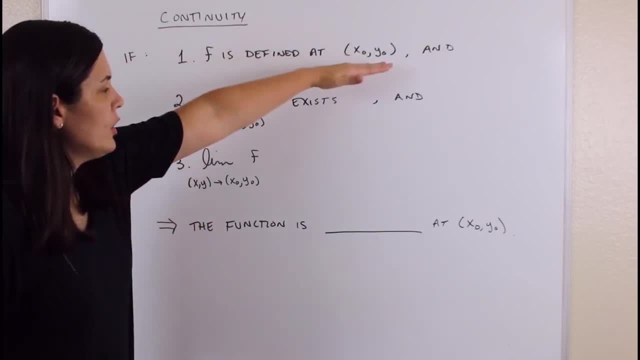 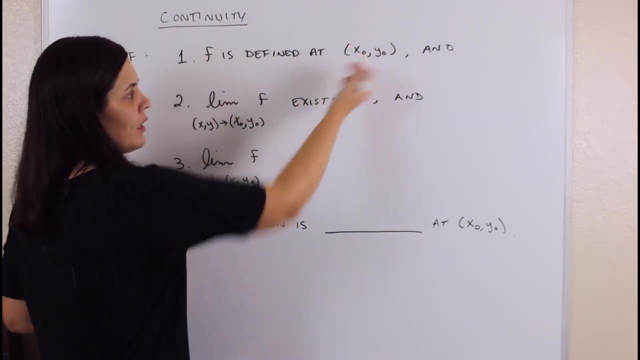 reason through. right now, The function is defined at the point. The limit exists as you get close to that point. Number three is that the limit is the number you get when you plug in 0.5.. All right, So you said you're going to get 0.5. 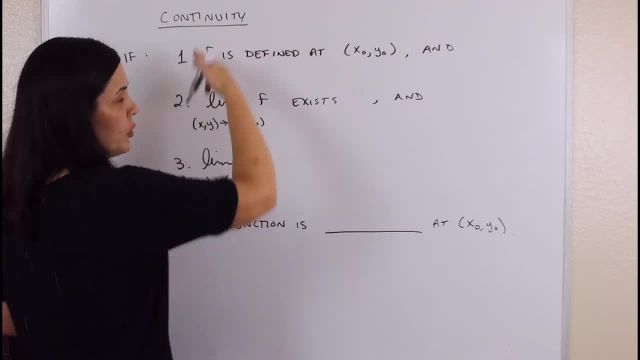 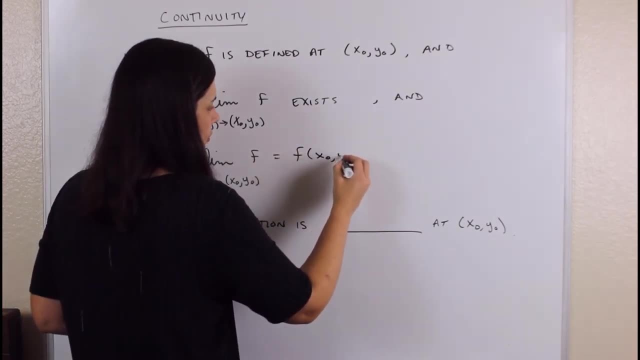 So the function is defined at this point, or this f value, this part 1, when part 2 and part 1 match up, is part 3.. So when the limit of your function equals the actual function value, then the function. 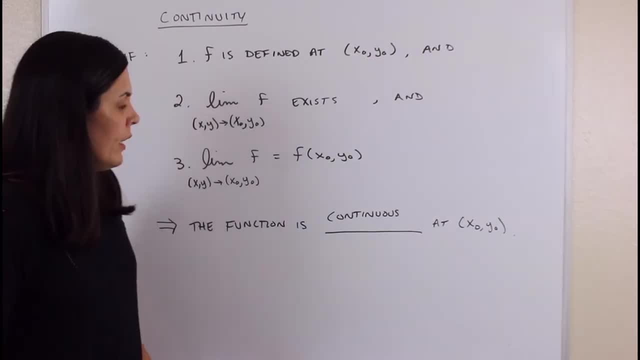 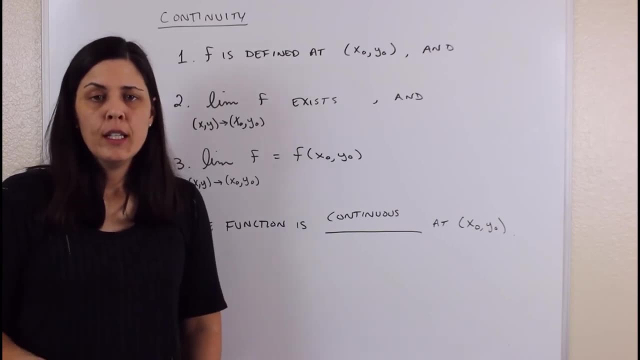 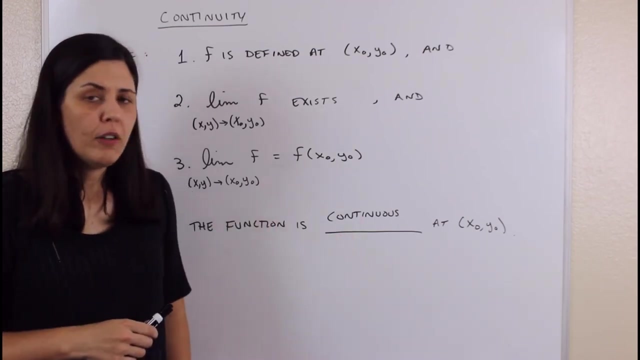 is continuous at this point. OK. So when we're talking about continuity of a function, we're kind of interested in where it might be discontinuous. exclude those things and then you say, okay on this domain, then the function's continuous. 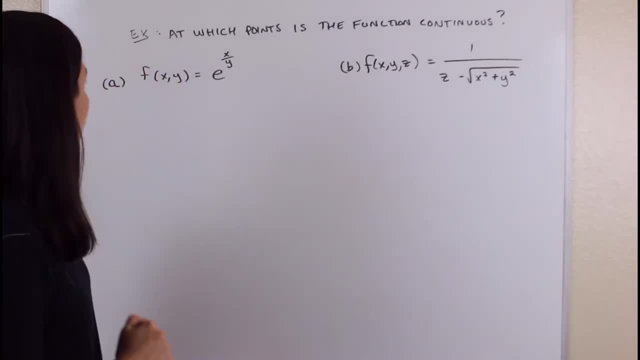 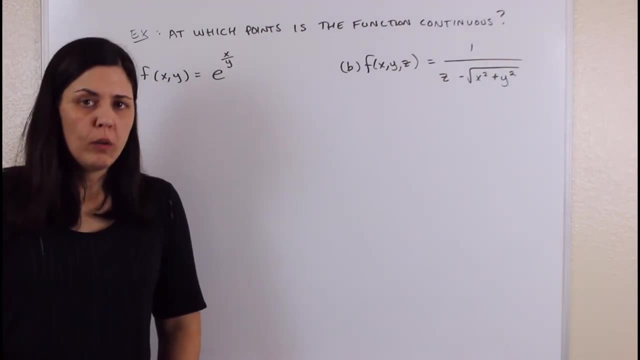 So let's try out an example. All right, so at which point is the function continuous? I have two different functions for us to look at here And you kind of want to just think about what would cause a problem, And the problems are fairly consistent. It's either like dividing by zero. 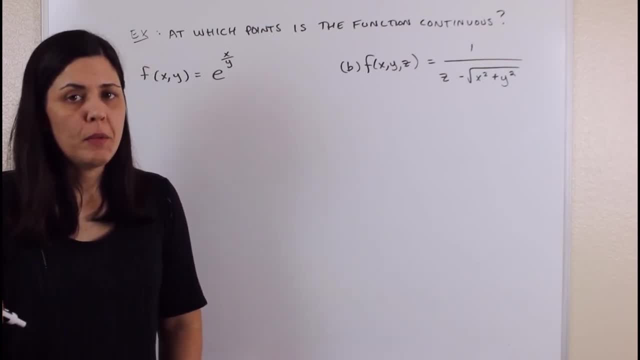 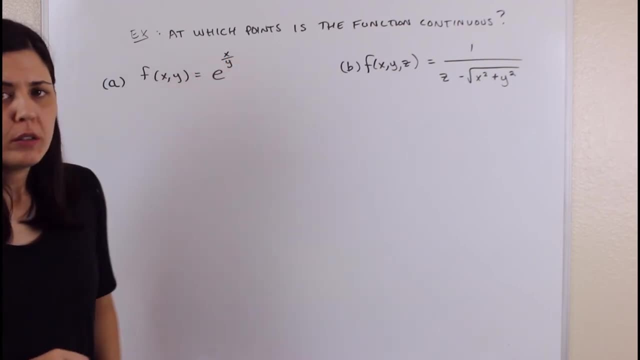 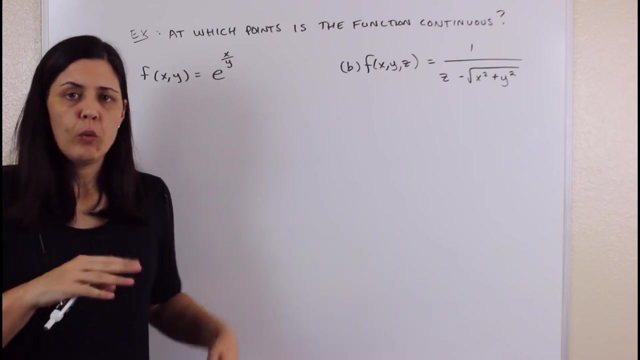 because it's undefined, or square roots of negatives, because that's imaginary things like that. So function a here, f of x, y is e to the x- y power. okay, So e the natural exponential function, e to the sum power that's defined on all real numbers. So e to sum power. 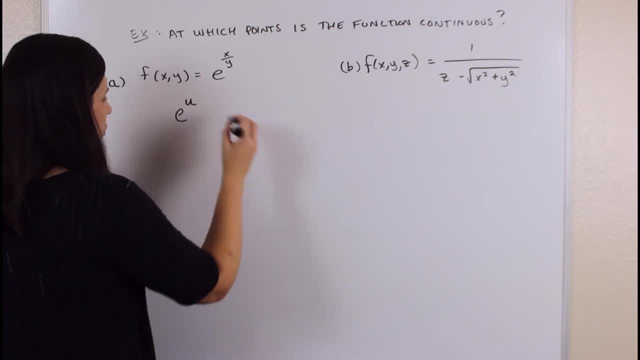 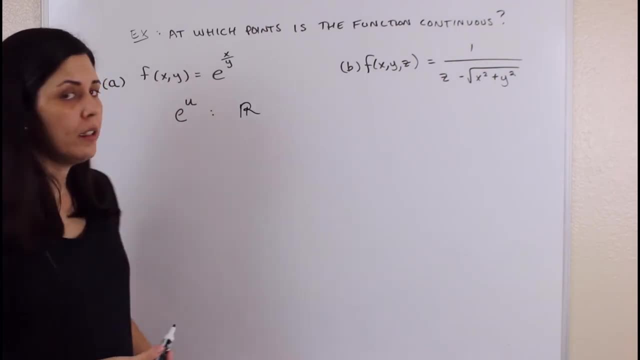 if you want to just sort of break this into two parts, e to the u, the domain is defined everywhere, So it's everywhere, all real numbers. You can plug in anything into that function. Now, this function, this power, this exponent, if we break that down- x over y- this has a problem. We cannot. 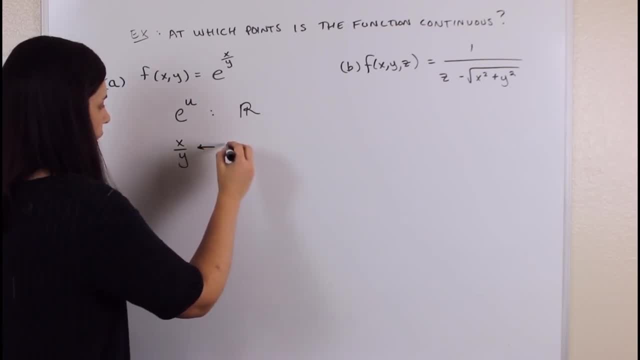 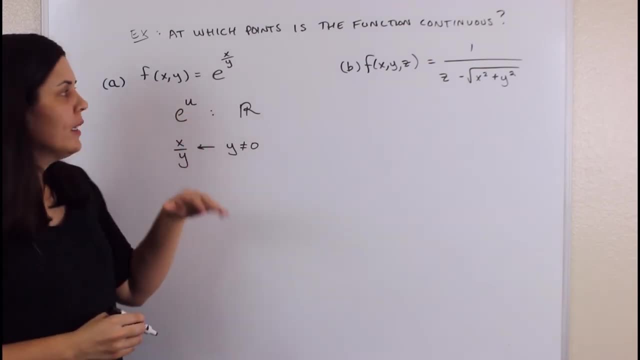 divide by zero. So this would be undefined if y was zero. So we want to make sure y is not zero. So if I kind of put these two things together, the only real issue is y can't be zero. So this function is continuous everywhere y is not zero. So notice, you're plugging. 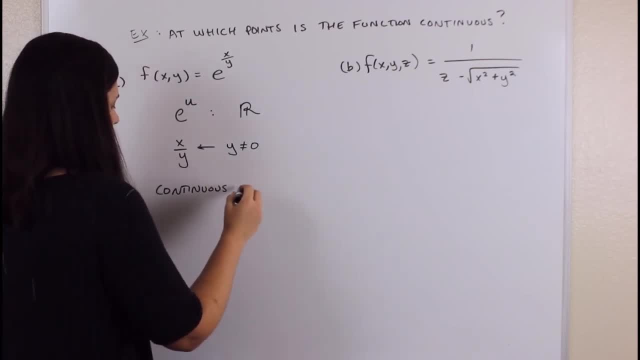 in for both x and y, So you can say continuous on this set. So you could say the squiggly braces for the set of all x's and y's, So all x, y values, And then as long as, or this: 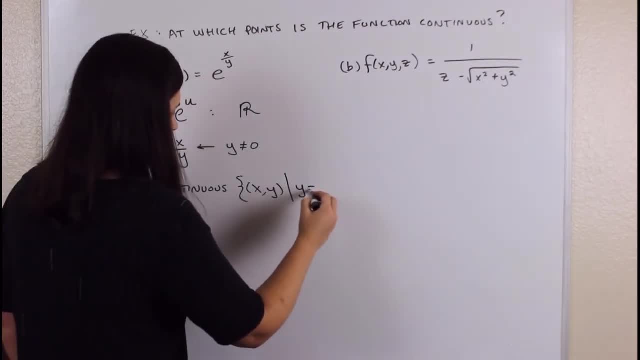 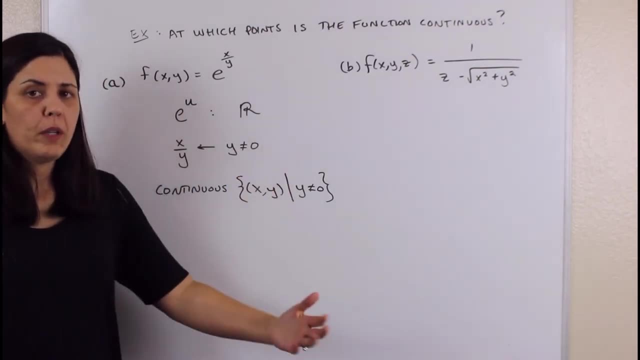 line actually means such that, such that y is not zero, And you can say this a few different ways, but that's essentially the same thing here. It's continuous everywhere, as long as you don't pick y to be zero. That's the only problem. So this next one. here we're going. 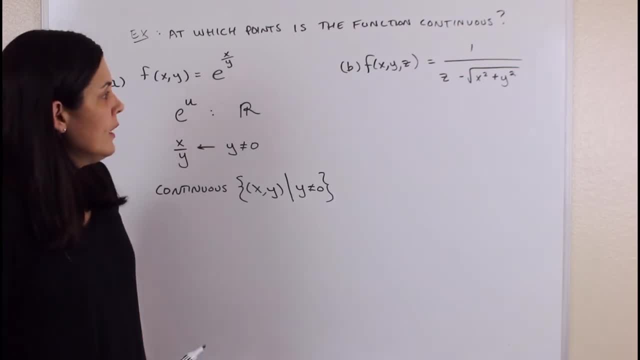 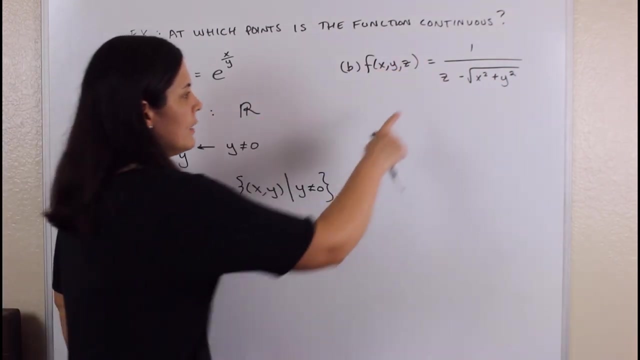 Notice it's actually a function of three variables. So just for reference, if this has three inputs, your output has to be something else. So just so you're aware, on this one the output would be another letter, maybe like w. So f of x, y, z equals one over z minus square root of x squared plus y squared. 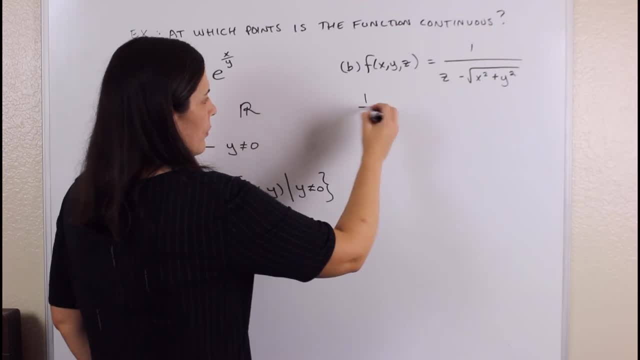 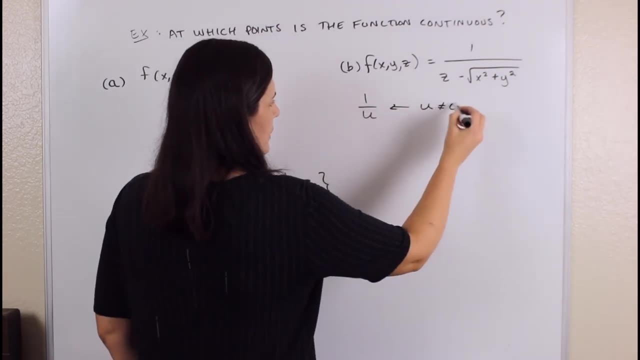 So the big picture here is that you have one over something. So this would be problematic if the denominator is zero. So on this one we have to make sure the bottom is not zero And then within the denominator we have a radical. 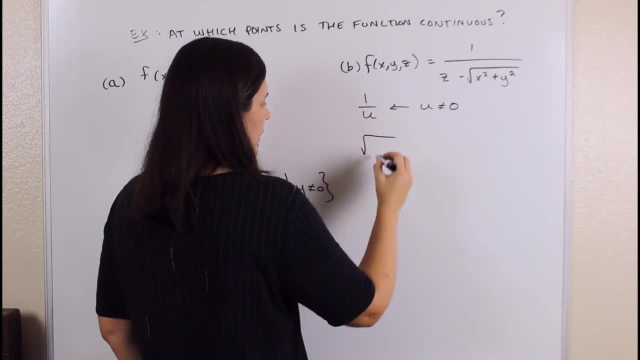 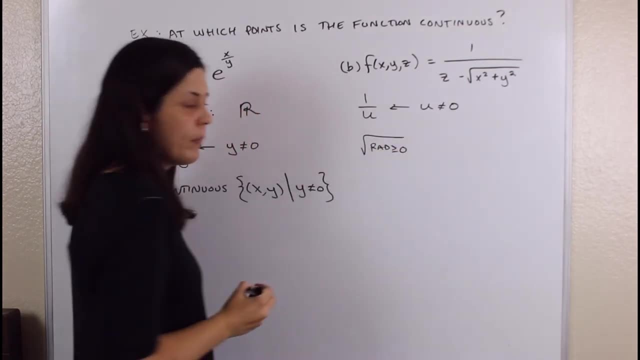 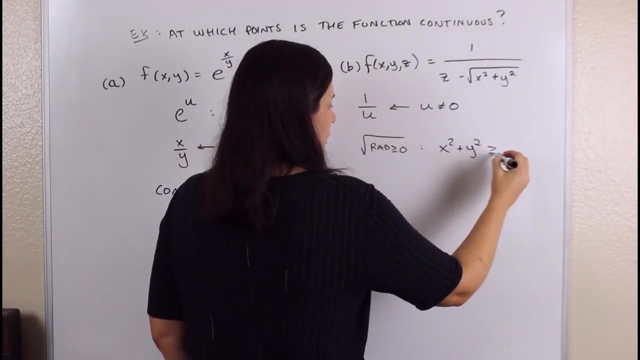 So with any radical we have that the radicand has to be zero or more. So we'll say the radicand has to be greater than or equal to zero. So we have to sort of put these together. So on this one, that means x squared plus y squared has to be zero or more. 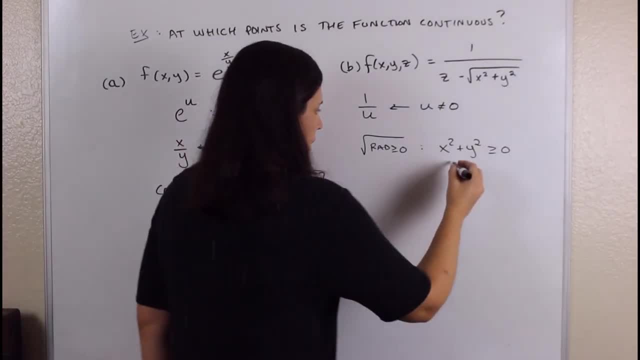 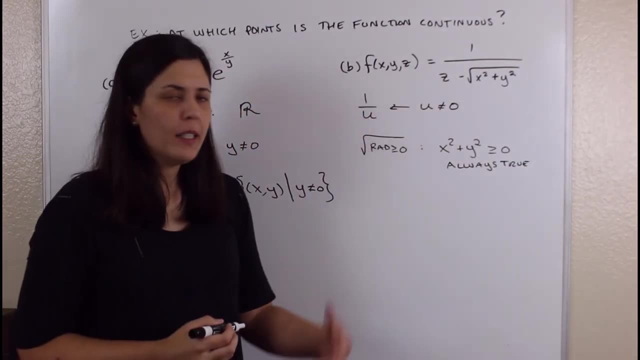 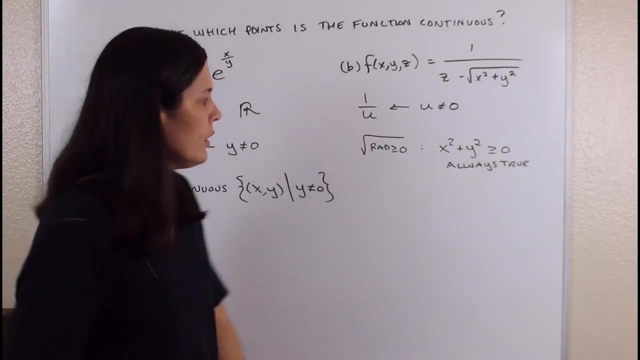 Well, there's nothing really to do here, Because right Here, on this one, this is always true. So that's nice That one's always true, because if you square anything negative or positive, it's going to turn positive, And then when you plug in zero, you just get this equals zero.